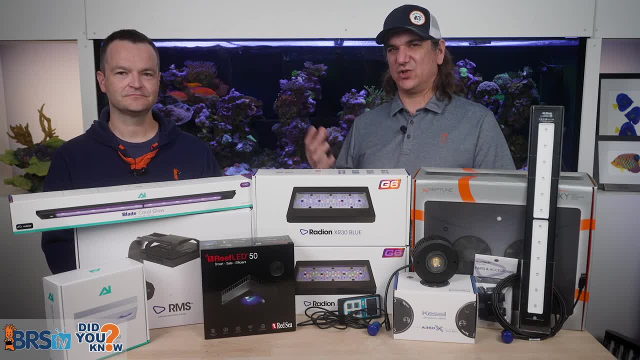 But it doesn't say that on the box anywhere. So how do I transition that without knowing and having to go do an enormous amount of research? Well, one really easy way is actually: just look at the watts that they draw out of the wall. 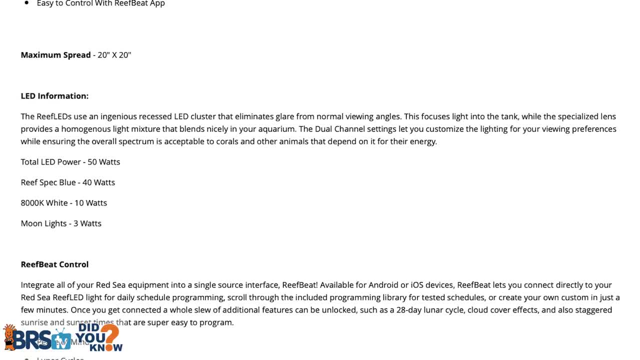 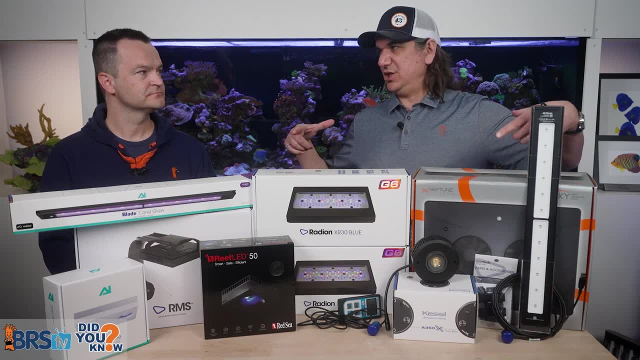 You can just go look at the product description and it'll tell you how many watts it draws, And I'll get you really, really close. And I'll give you an example. We're gonna talk over just a two foot area here. 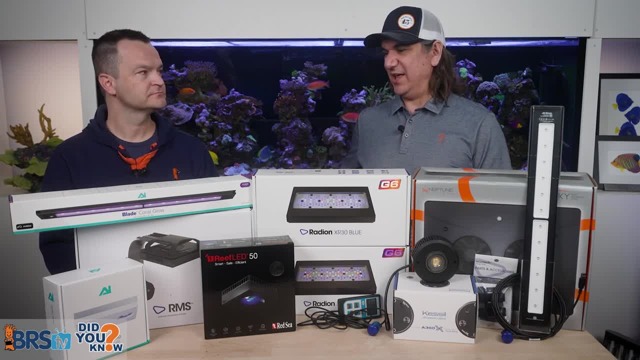 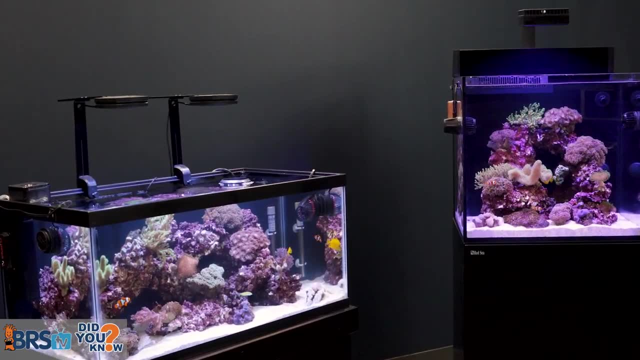 but in that 50 to 100 watt range at the wall we're talking about Kessil A360s, the ReefLED 50s, the AI Primes, even like a couple of blades, anything in that range of a total. 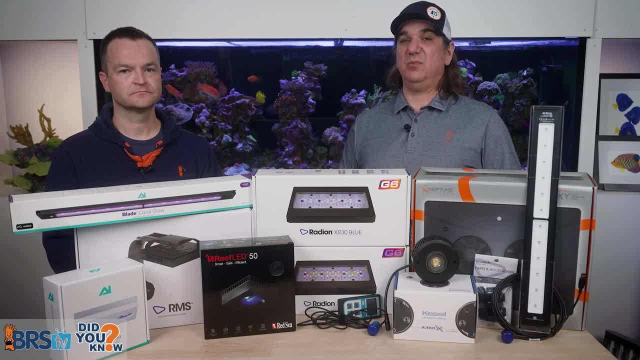 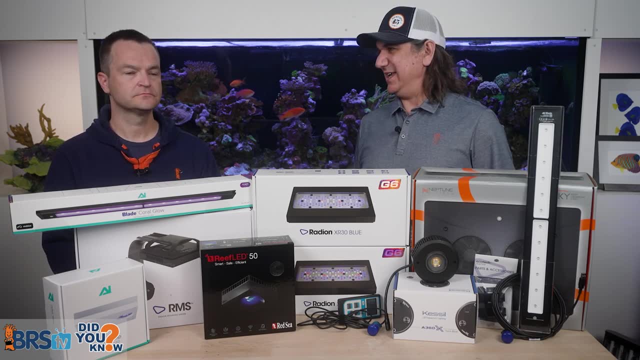 of a 50 to a 100 watt range. that is going to be your sweet spot. now for LPS, Yeah. and so what if I wanted a like a mixed tank though, which is gonna have some spots in there in the SPS range? 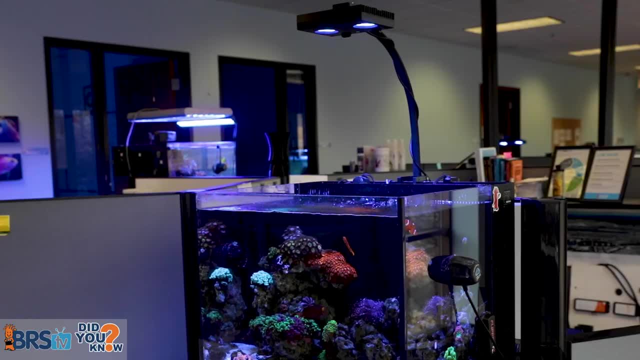 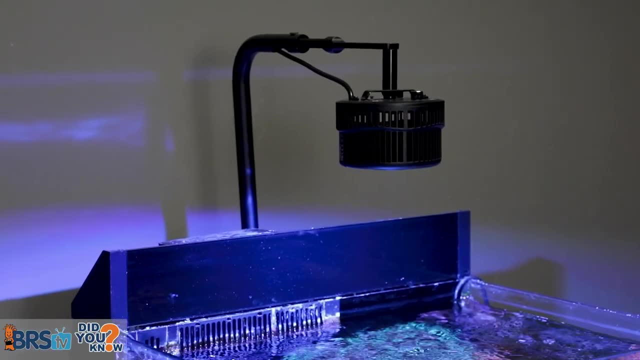 Well, now I'm looking at 100 to 150 watts. This is like your Hydra 32s, your XR15s. This is even like the Kessil 500X. we're stepping her up In that range. now we're doing these mixed tanks. 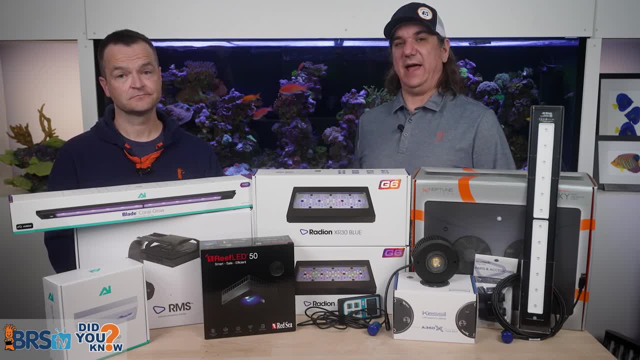 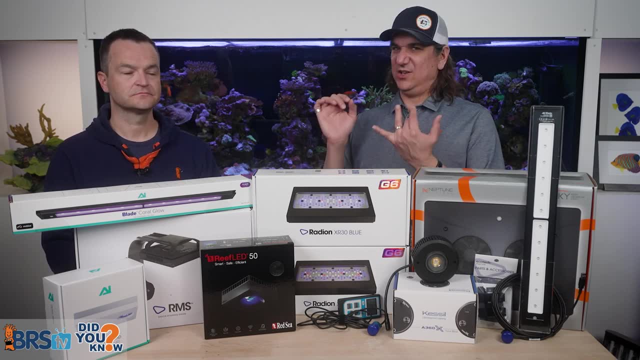 which are probably amongst the most popular. But what if I wanted to go to SPS? Now I'm breaking it into a totally different category of about 150 to 200 watts at the wall. This is your XR30s of the world. 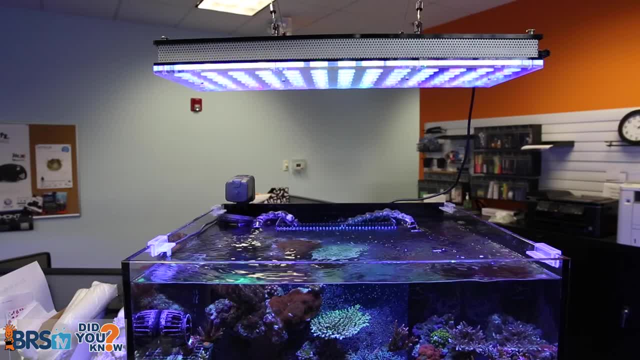 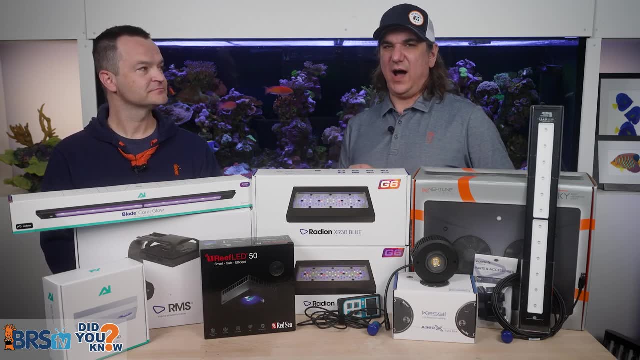 This is, you know, your big, huge panels like Orpix. I think even the Sky is probably in that range. yep, So now I can actually shop just by looking at the watts. Now, the watts, you know, won't get you all the way there. 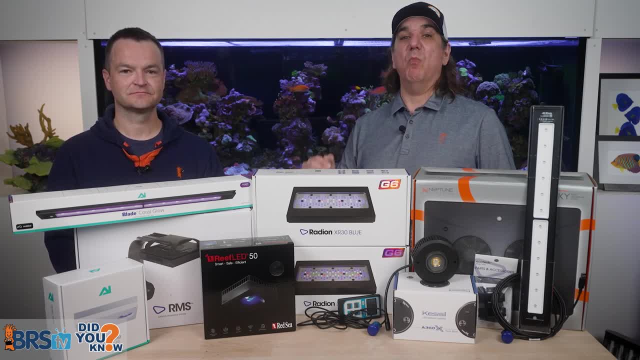 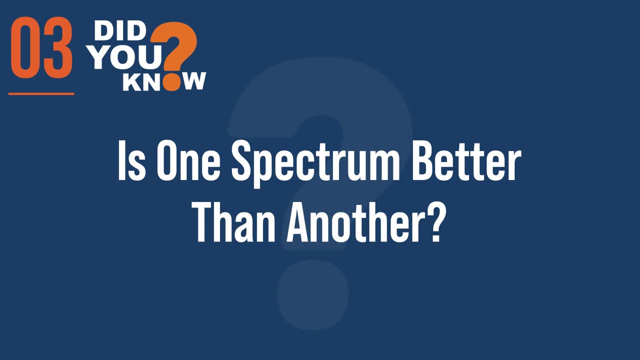 but it's a way, way, way better option. And now I don't have to buy more than I need, which makes it easier to find value. Number three are the spectrum offerings better. from one fixture, one light to the other. 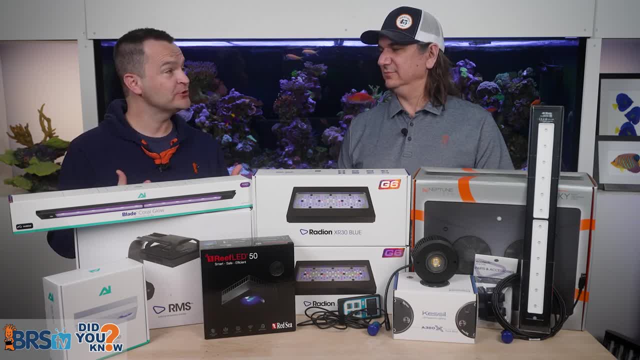 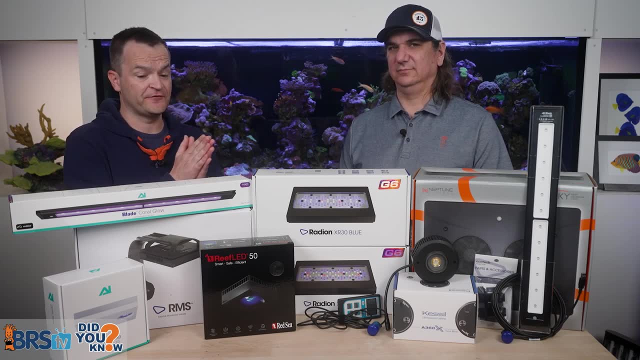 Absolutely, yes, 100%. But how will you know the spectrum of one light versus another? I mean, just how are you supposed to know that? Well, the general rule of thumb here is: when you're looking at the spectrum offerings- and you can find these oftentimes on the box. 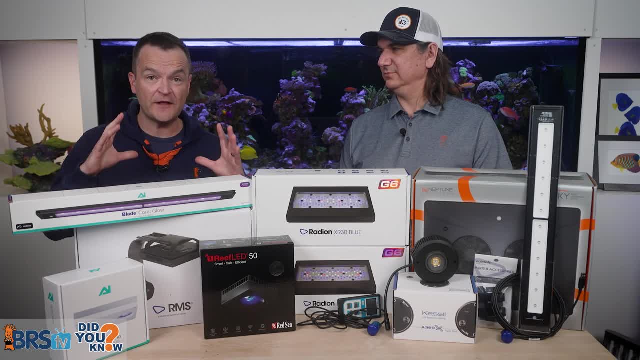 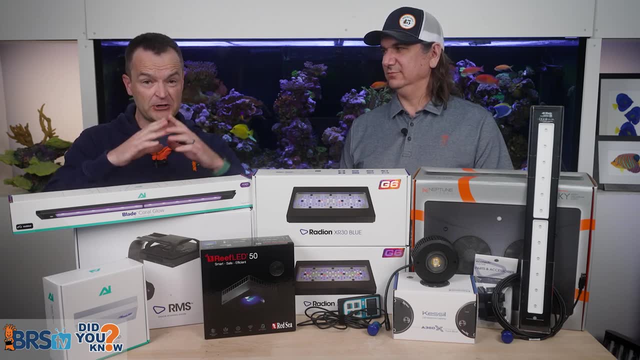 you can go online and you can see a spectrograph and you can see exactly what the spectrum is. But when you're looking at that spectrum, you're looking for the blue. You're not looking for little tiny blue peaks, but you're looking for a wide swath. 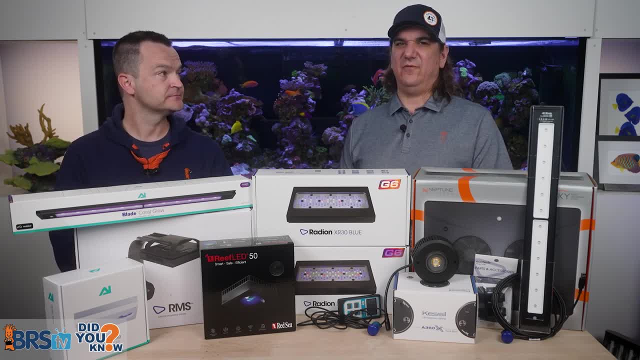 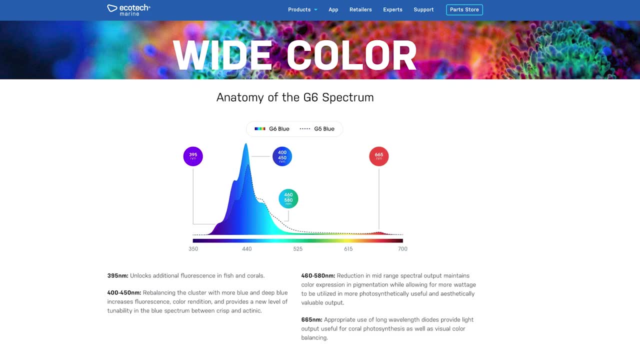 that the light covers a majority of the blue light out there. Yeah, in fact I would say: go to the website, go on the product page, go wherever it is and find out like. just look for it If it's a tiny little like peak. 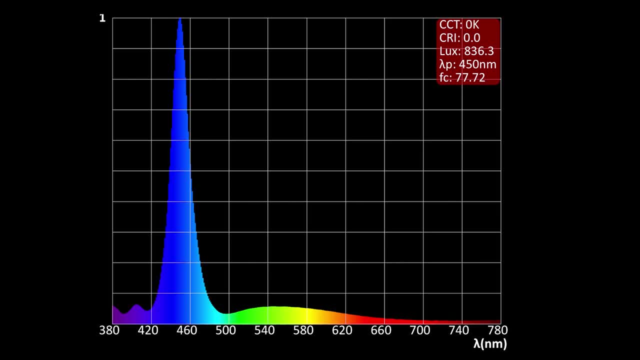 that looks like a laser beam or the Eiffel Tower. this probably isn't the best one. If it is a big, wide blue band, it probably is amongst the best ones. There is a couple of reasons for that, In fact. I'm gonna go one more further. 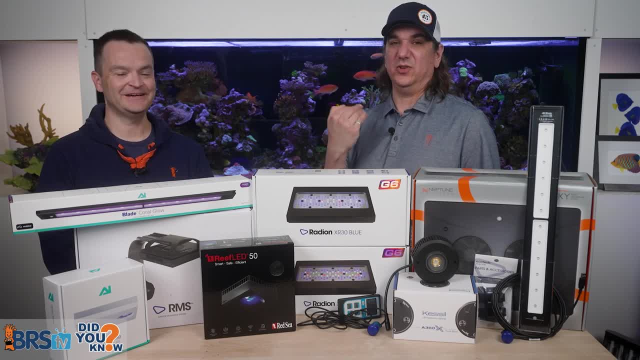 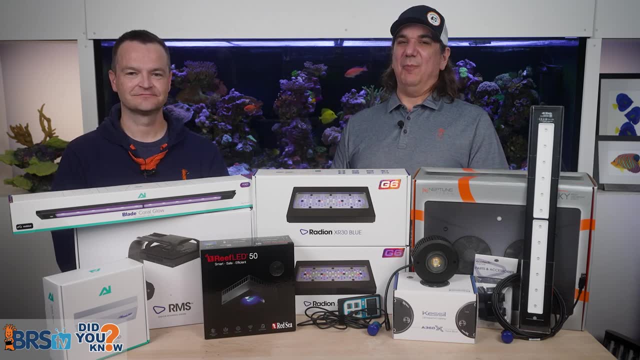 If you can't find this data on the website, just skip it all entirely. Either they don't know or they don't wanna tell you- I don't know which one it is- but either case just skip it. But what you're looking for is this thing called. 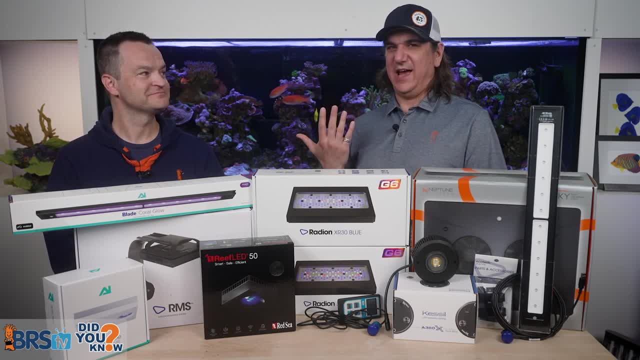 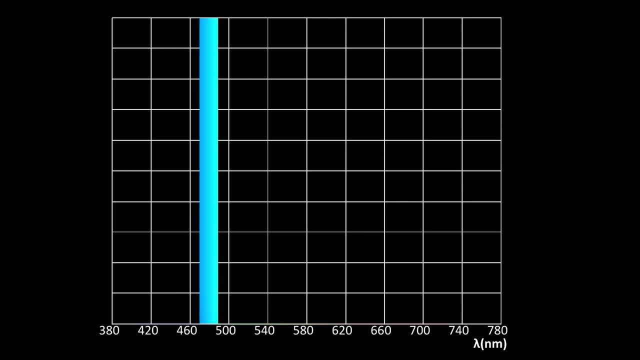 it's a mix of like nerd talk of nanometers and then normal talk of just color. So what you're looking for is light blue, which is around 470 nanometers. So light blue, 470.. You're looking for like a deeper blue, which is like royal blue color. 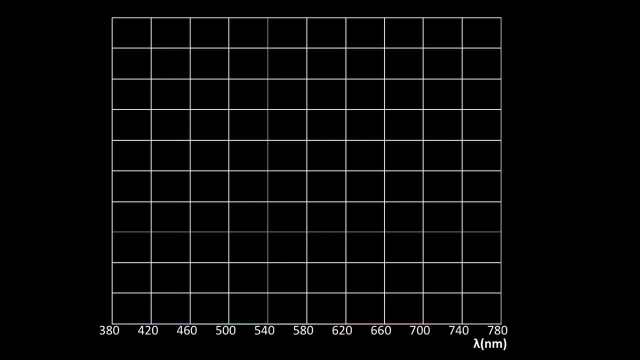 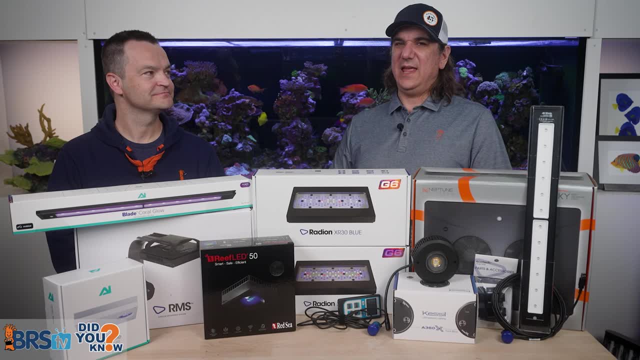 which is about 450.. And then you're also looking for violet, which will go all the way down to like around 390.. And these are just kind of you know, rough areas Well, so I'm now covering a wider span. 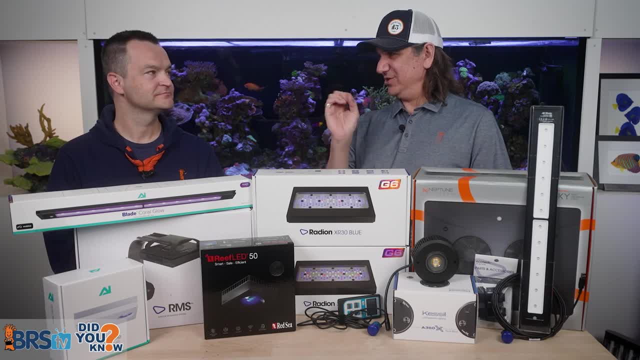 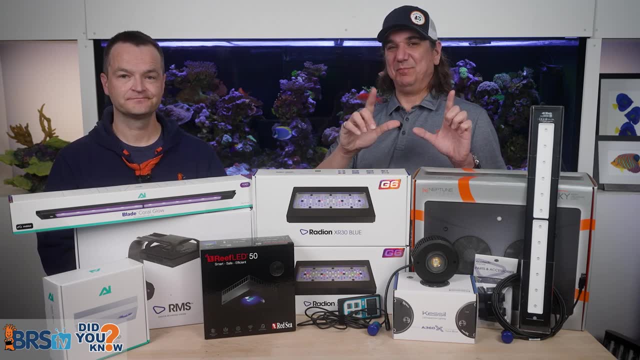 Not only will that show up in coloration of the coral, cause they have those colors that actually show, but there's also biology in the sun. So the sun actually covers that whole area right, It doesn't have just a little weird peak. 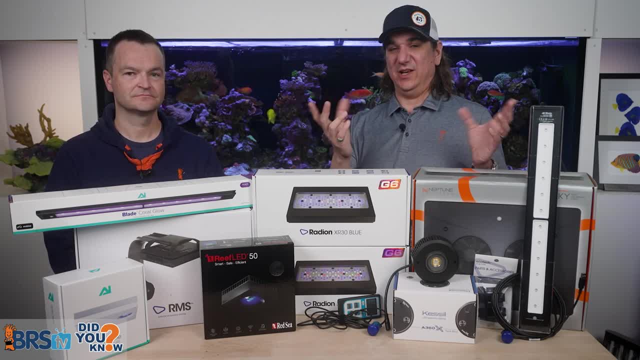 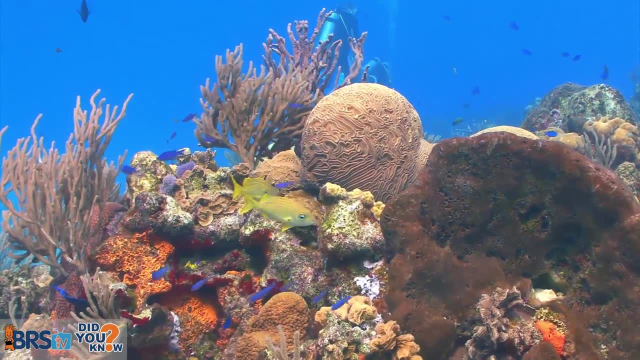 in there. It covers the whole area. Your eyeballs can't really see it in many cases, but why does it matter? Cause first the sun. these things evolved around the sun And, as we know, biology doesn't make a whole lot of mistakes. 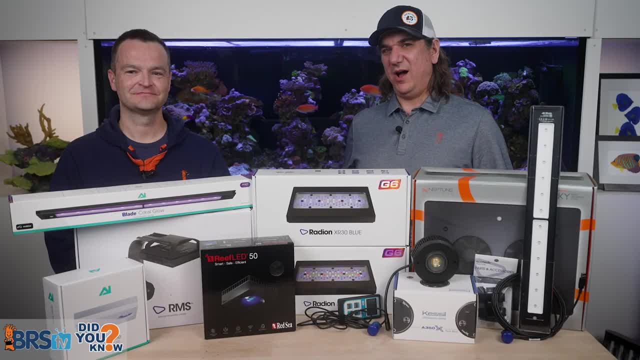 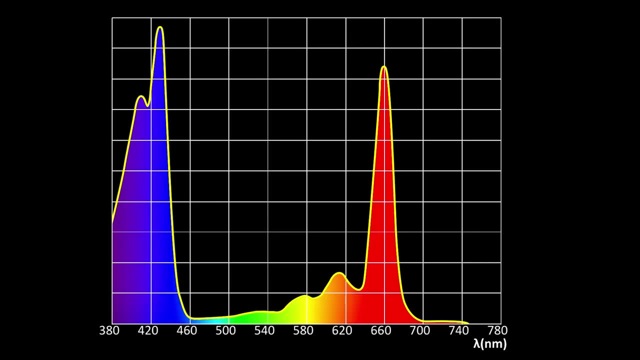 over a long period of time, Very, very few. But the reason why that biology is is you call it, you know, violet light. What we'll call it is chlorophyll A light, So this is where chlorophyll A within the zooxanthellae. 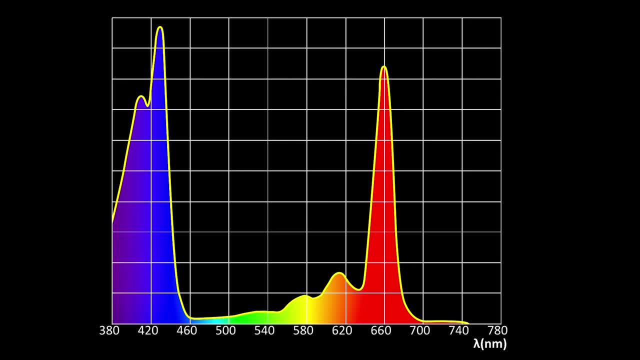 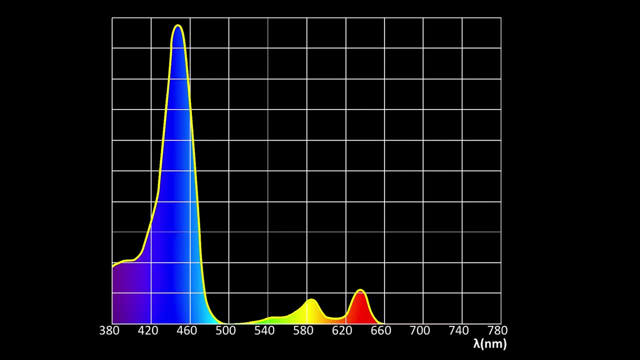 actually absorbs like light the best. It's in that violet range. You may call it like blue light, but we're going to call it chlorophyll C2 light, which cause. that's where chlorophyll C2 actually absorbs lights the best. 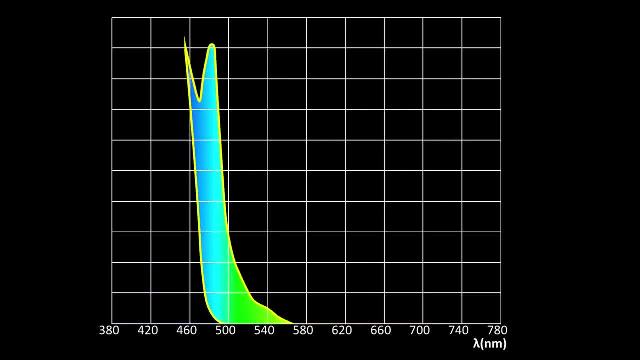 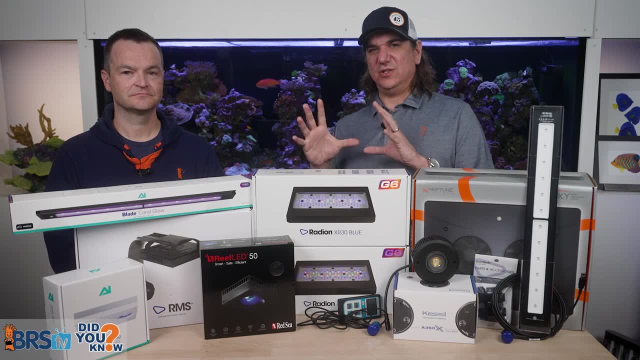 And you may call it light blue, but we're going to call it pridininin light, or an area of the carotenoid zone. So these are the things of like the chlorophyll and the carotenoids is where they absorb light. 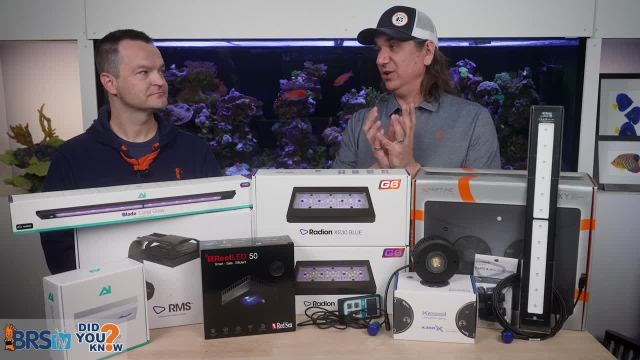 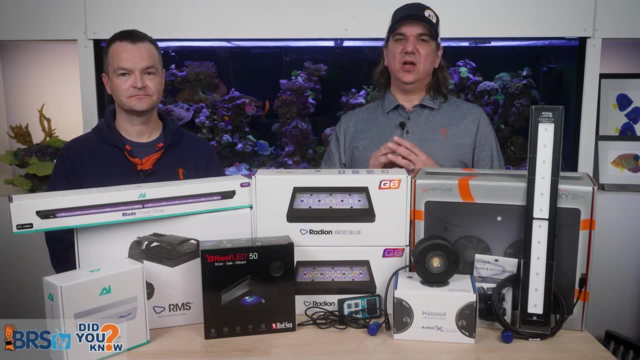 and then pass it and turn that light energy into glucose and glycerol for the coral. So if we just provide one of those things, this coral is going to have to wildly adapt its biology. So we know that the sun. we know the known biology about chlorophyll and carotenoids. 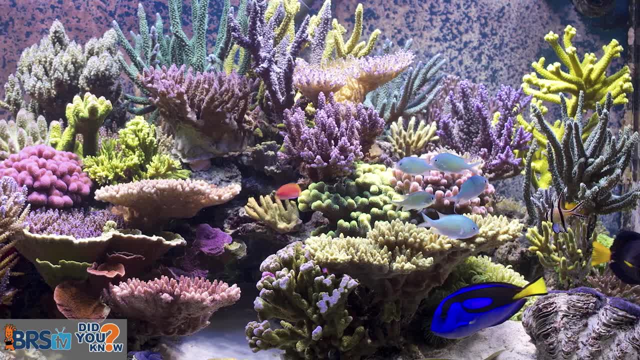 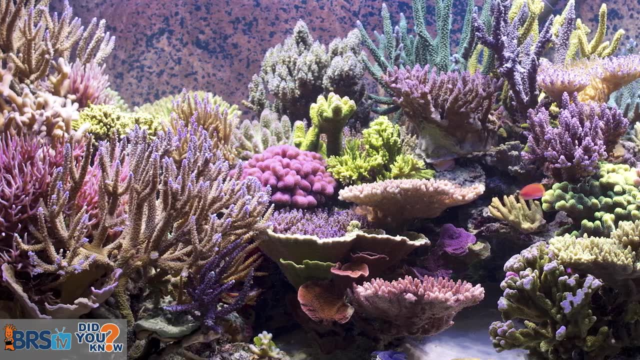 but we also know is success, which is all of the most successful lights out there that produce the most successful tanks out there. all have big, wide blue bands. Now, here's the good news: There's many, many options out there today that have wide blue bands out there. 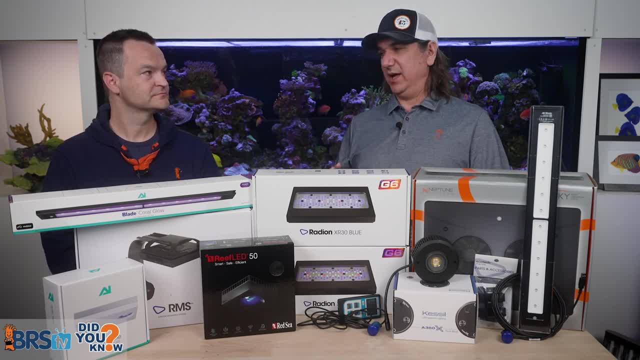 And some of them are even adjustable. So like, for instance, if you picked up like a Radion, it will have a big, huge blue piece. It will have a big, huge blue piece. You can actually tweak it down just a little bit. 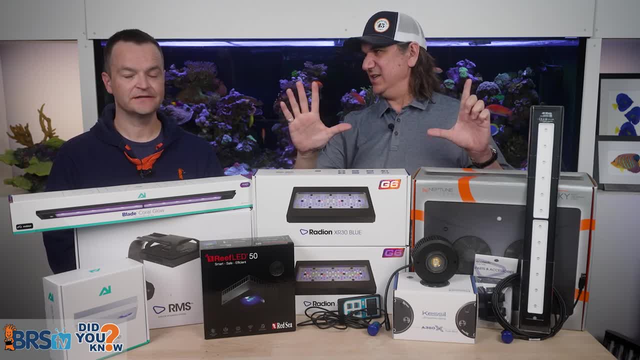 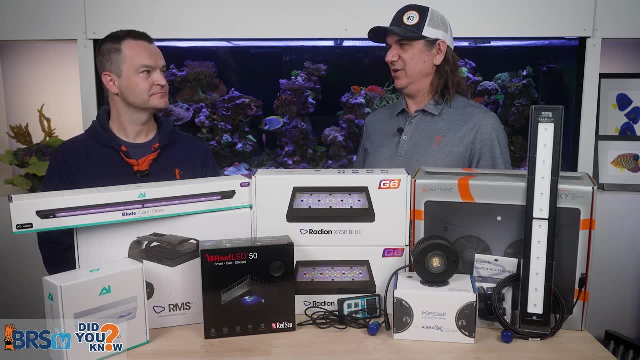 and it becomes wide. but it gives you the ability to change those colors. So it actually has all of that stuff down there. but there are lots of options to have it out. But let's pretend you know what I'm watching- this video. 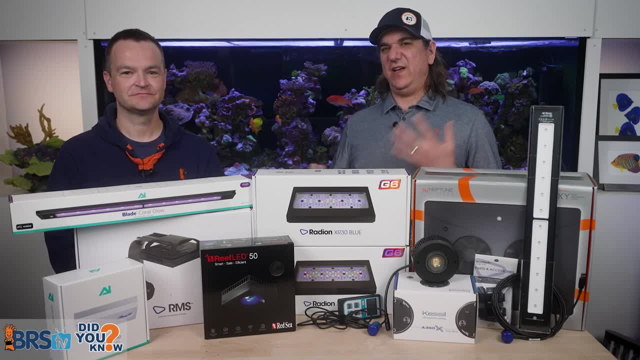 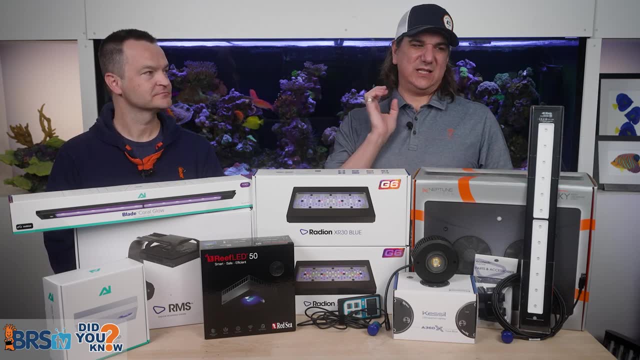 and I realized I bought the wrong thing. Now, when I have the Eiffel tower, you can actually fix it now with, you know, throwing stuff like the blades and stuff on the side or really anything. I will say I specifically say the blades are fixing it. 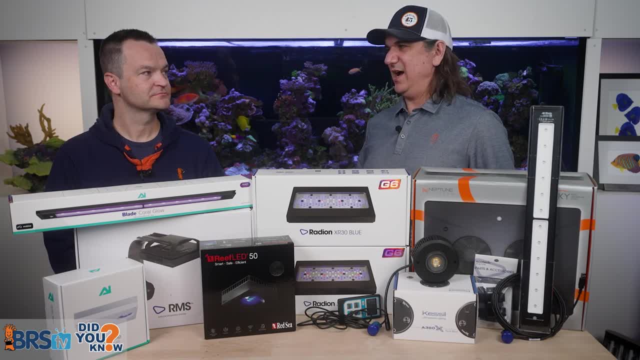 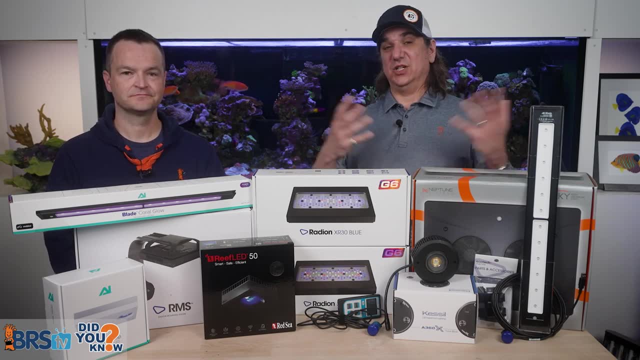 because there are other light strips out there, but most of them are actually just adding more of the light you already have. you know which is this like Eiffel tower thing. So we don't really want more of that, We want to actually expand it. 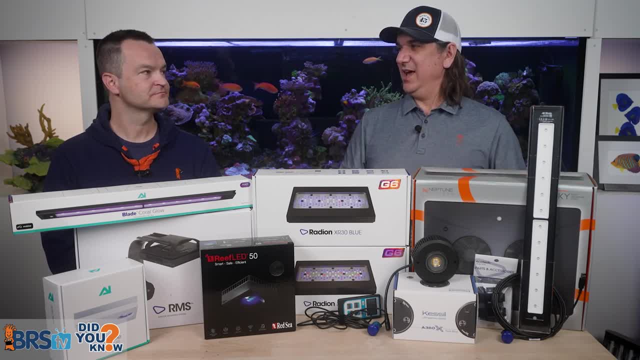 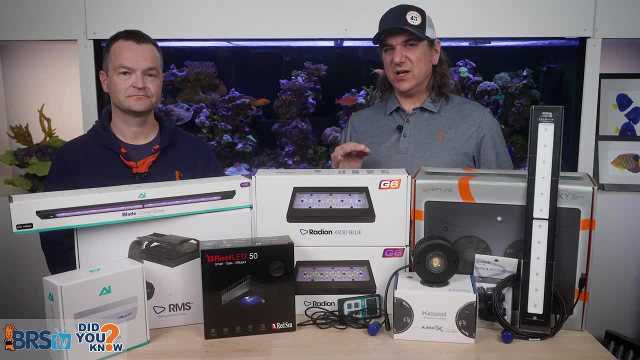 And then options like the glow gets into that chlorophyll A zone and the grow gets into that light blue zone or carotenoid zone. So spectrum does matter. Now there's a whole lot of talk here but like basically all it's telling you. 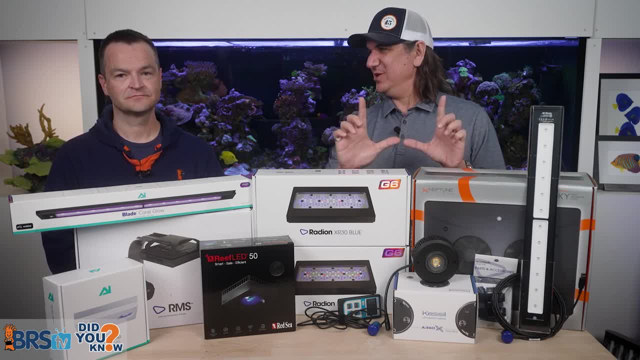 is: go look at that chart. I'm looking between 390 and 470, if you've got numbers there, or I'm looking if I don't have numbers. I'm looking between violet and light blue And that's how I know I've got a light. 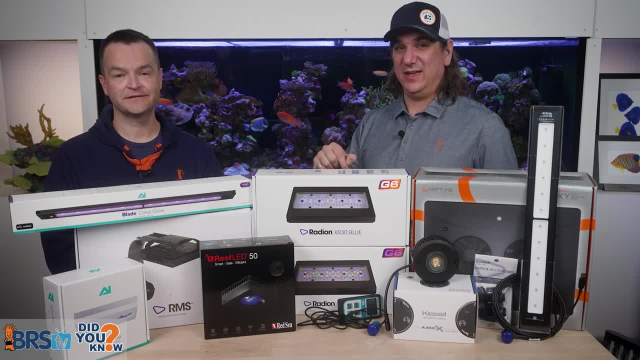 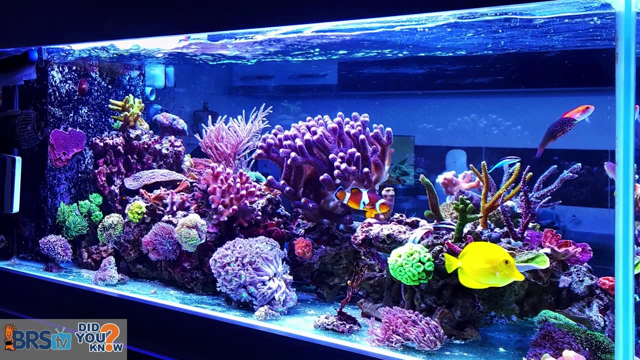 And right here I'm gonna tell it to you: buying it right to begin with is way cheaper than fixing it later. Number four: does size of the light matter? Yes, absolutely. The best approaches here are going to blanket the tank in light and reduce shadows. 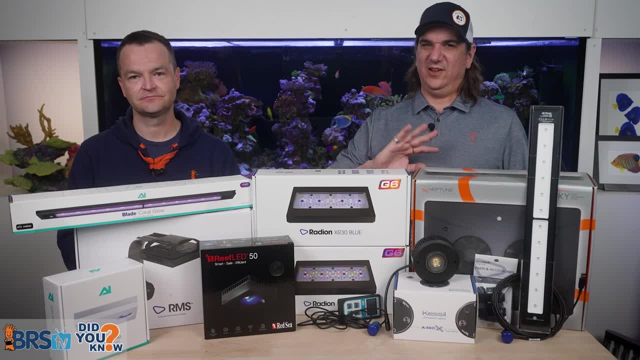 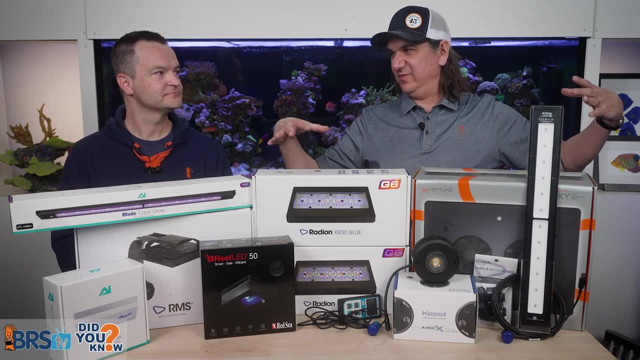 This is probably one of the biggest follies, as we went from like halides and T5s and stuff to LEDs is visually, your eye can't really tell. you know a tiny little light that has a fairly wide angle. It looks like it's illuminating the tank. 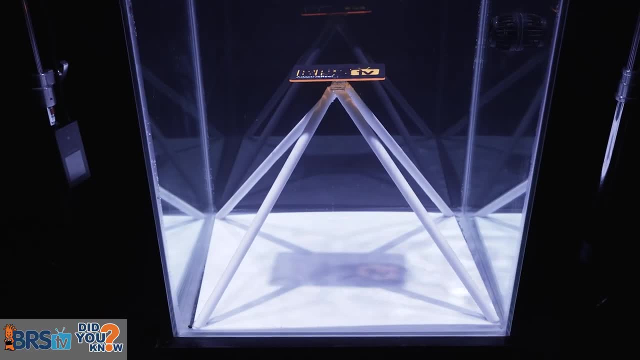 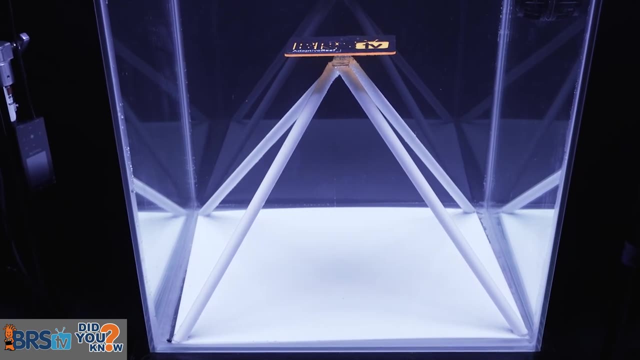 but if you actually get the meter out you'll find out that it's just like everywhere. it's just shadowing, Like there's no way around it. A little light like this is easily shadowed. Light's not getting through. But if I have a big, huge, giant light at the obstruction, 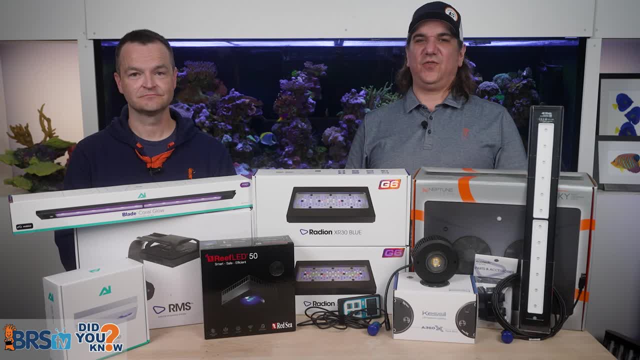 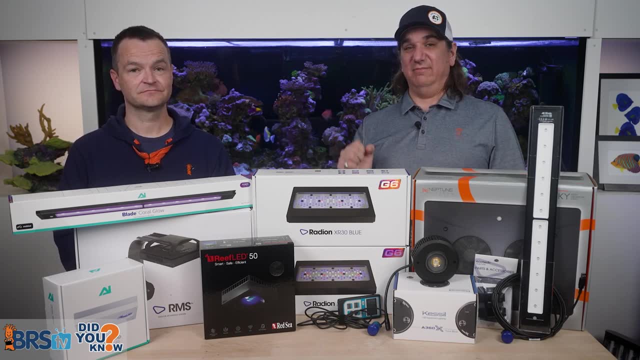 it hits it from both sides. It's just the way it is, And so, just for a reference point, we find that the shadows generally reduce the PAR by like 75%, And you'll just see that like you'll get these weird, abnormally shaped corals that, like one of them, grows. 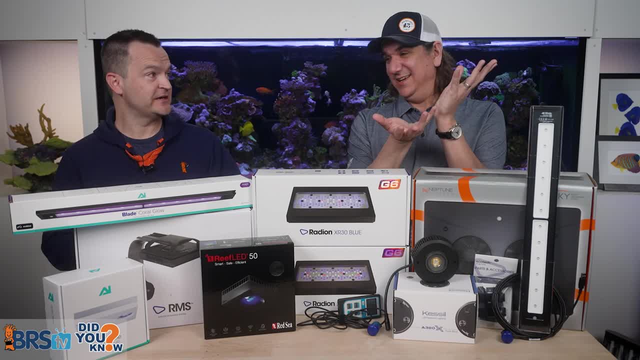 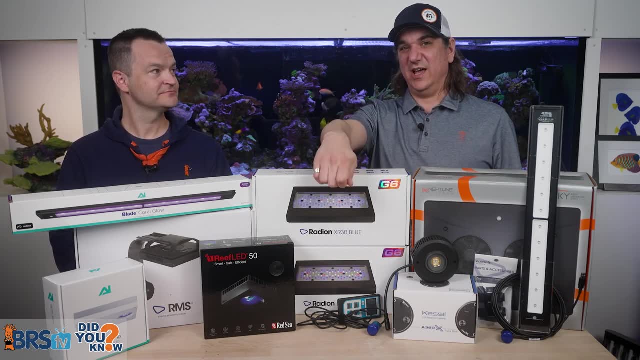 where there's light and the other one just doesn't. Yeah, it just doesn't grow right And then, yeah, it's like dead underneath and the inner shadows Cause if you put your PAR meter in there, where the shadows are, it could be like five. 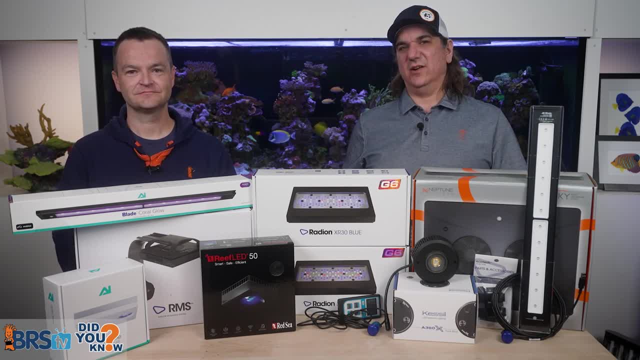 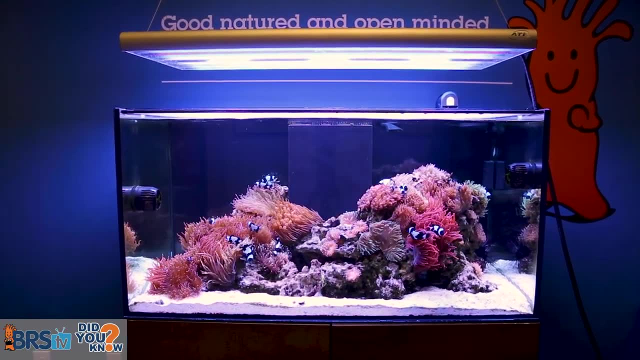 Yeah, So yeah, size definitely matters. but size doesn't have to be the only thing, Cause you could get a big, giant light like a big time. you know T5 fixture on the top. That's one way to manage that kind of horizon to horizon. 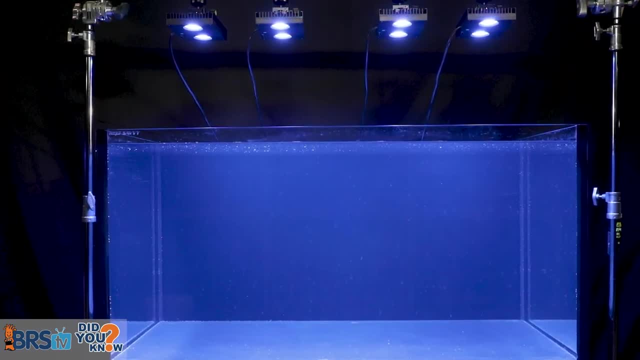 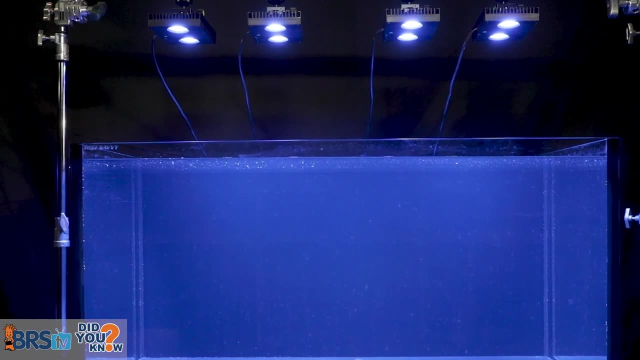 size matter conversation, There's another one where I can just get wide angle lights and I can space them about every 18 inches, which kind of blankets the tank Not quite as well, but also less obtrusive You can also take. well, damn it. 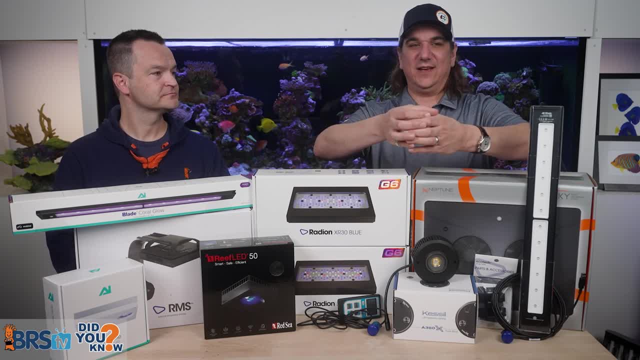 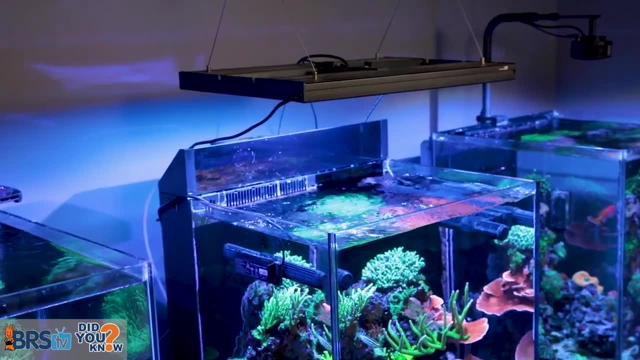 I already bought those like little pucks, And I hear what you're saying and I'd like to fix it. Well then, throwing fill light on the sides of them, you know, creating three point lighting that kind of matches- the sun and the sky- works really well. 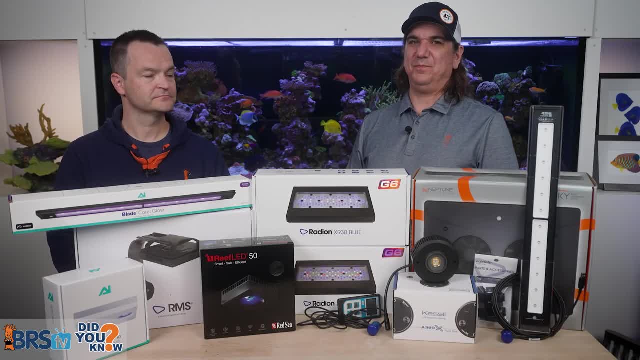 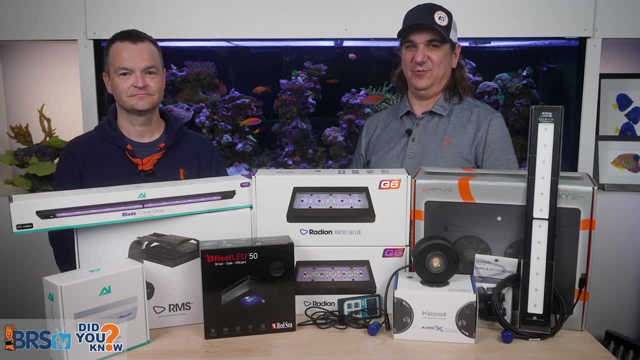 So this is the point where I wish, like if there's one point here I'm going to, we have a one point at the end, but I'm going to give you one right now- I wish that if everybody just heard this and we could just like embrace it and adopt it. 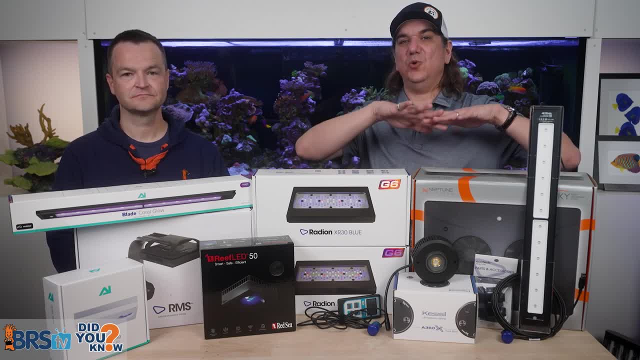 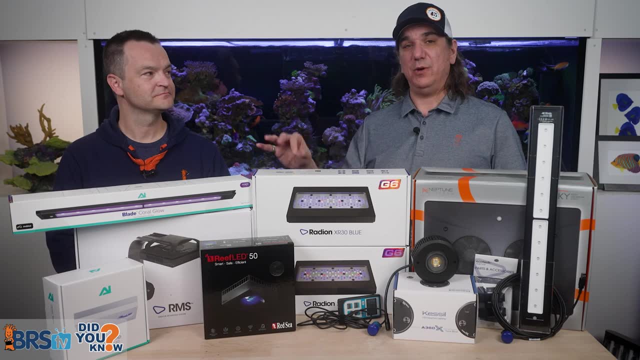 we'd all be so much more successful, which is we need to blanket these corals and light from all angles. If we do that, you'll be way, way, way more successful reefer, and it'll help you pick the right options. 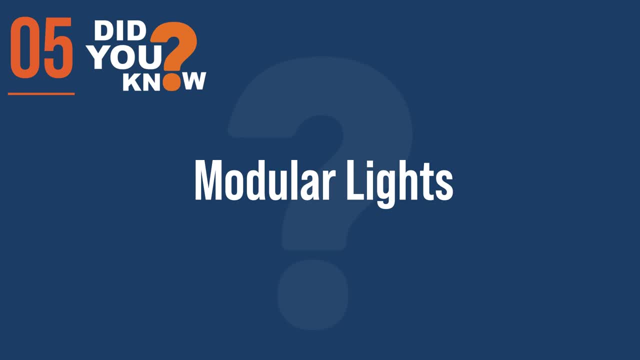 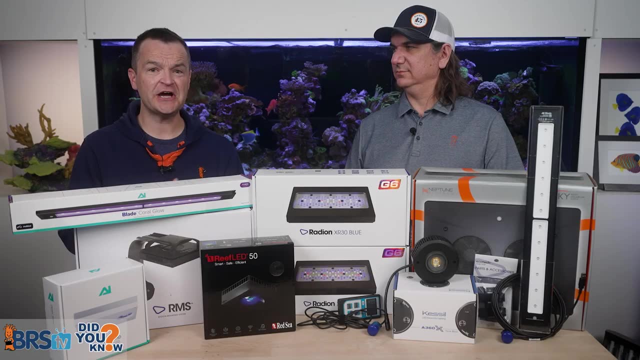 Number five. there are four approaches to accomplish what we just discussed, Each of which has benefits but work differently, And the first one of those is modular lighting. We're talking about things like the Kessels, Radions, Hydras, Mitras, Reef LEDs. 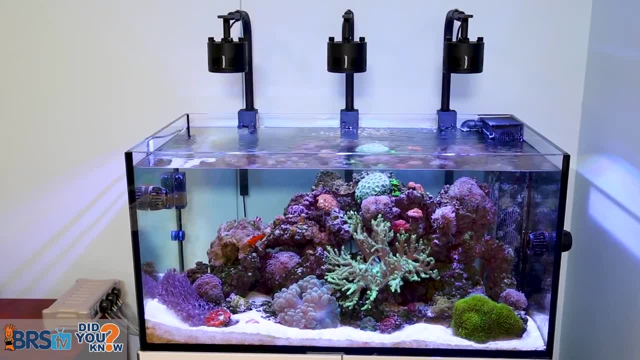 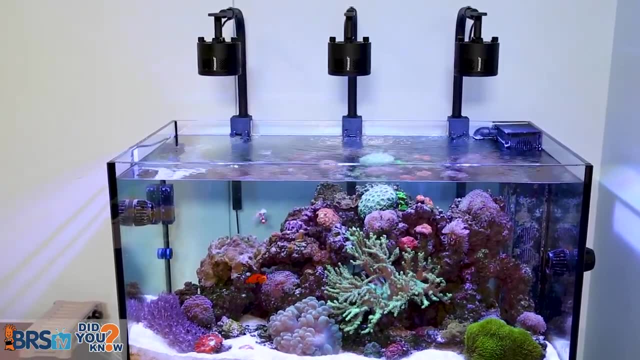 Some of those are definitely the most popular. These are generally smaller modules, right, And you space them between 12 and 24 inches apart, And these are great for a lot of reasons. These are like number one most popular, as picked by you guys, for sure. 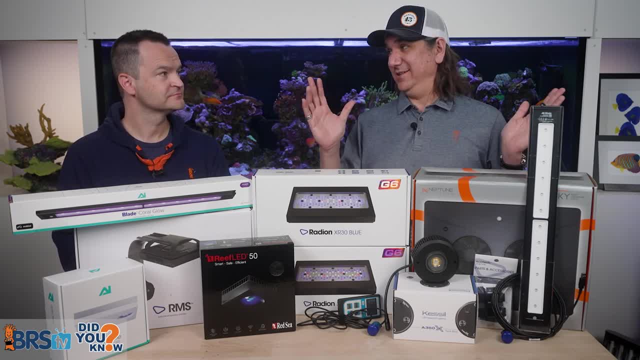 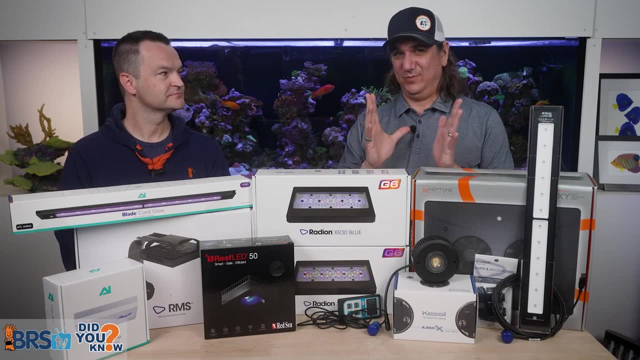 These modules. they're great because visually, man, they're really low profile. The whole top of the tank's open. I can get in there. The stores love them, man, because it's just one box on the shelf, real easy. 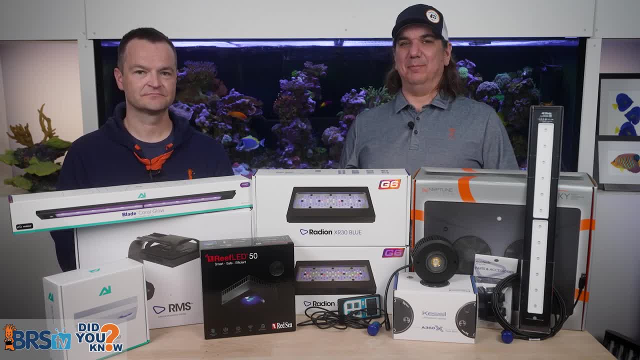 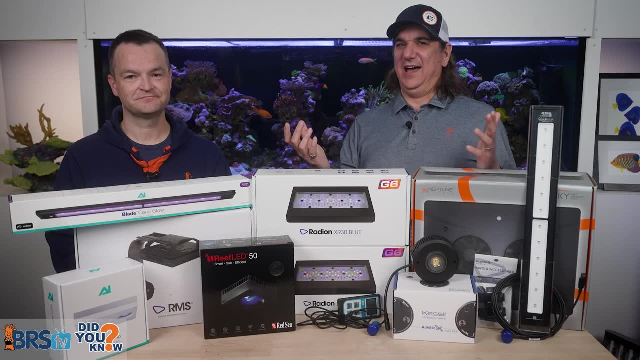 They're just really, really, really, really popular. I think the biggest fallacy, though, here is that we tell everybody to do them every 24 inches- at least the box does- But really, where people have the most success is when they're about like every 18 or 12 inches. 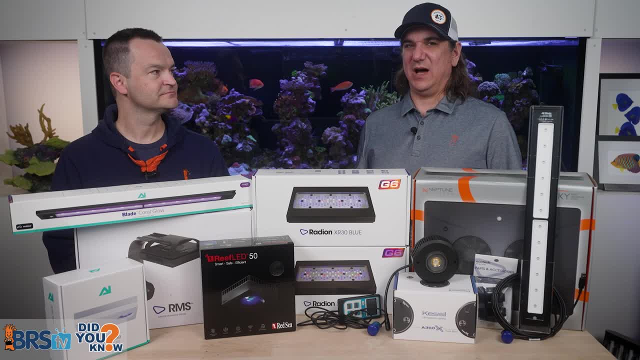 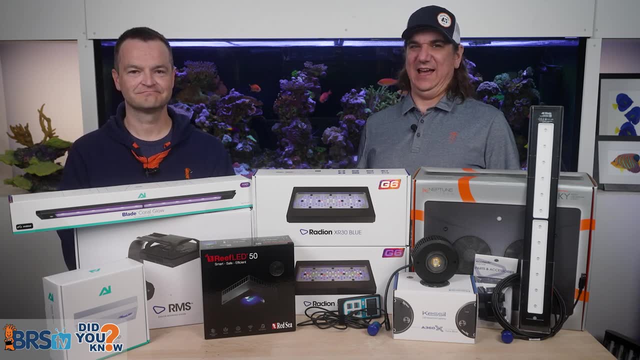 But I got to tell you one of the things that makes them probably the most popular is: these modules are really really easy to mount, And we've polled people many, many times And the answer is always the same: What's most important to you? 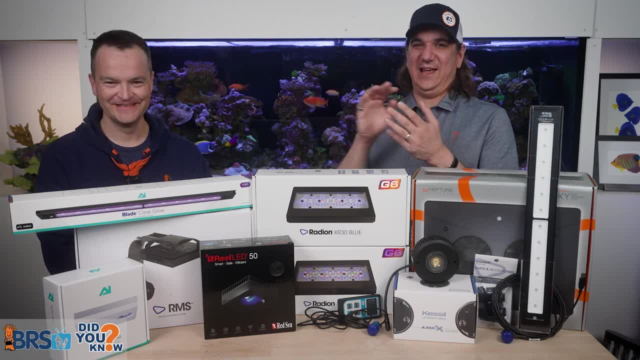 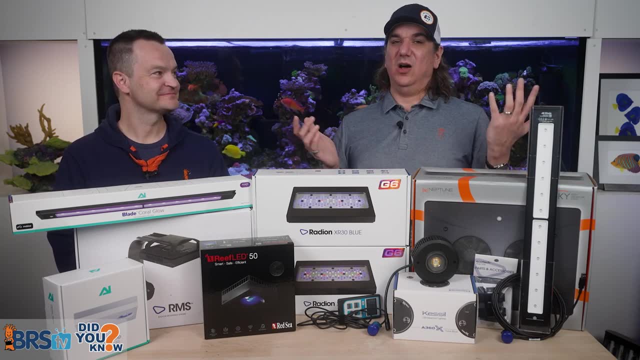 Is it coral growth? Is it coloration? Is it like 80 million things, And the number one always comes out- is easy to mount, And so these are easy to mount. Now, the only part of this is you know that you're not doing this as well. 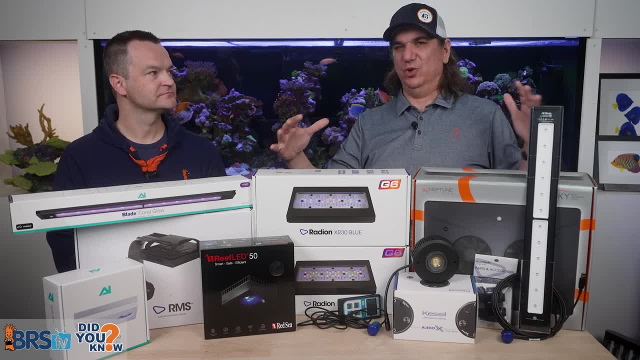 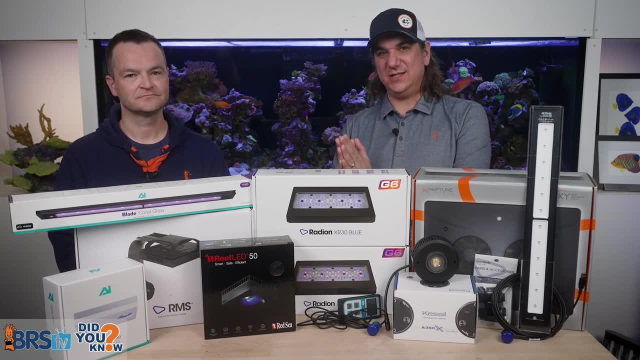 as a big blanket of light. So how do I make that a little bit better? And it's probably by spacing them every 12 to 18 inches instead of every 24 inches, And you will see this in every tank of the month. 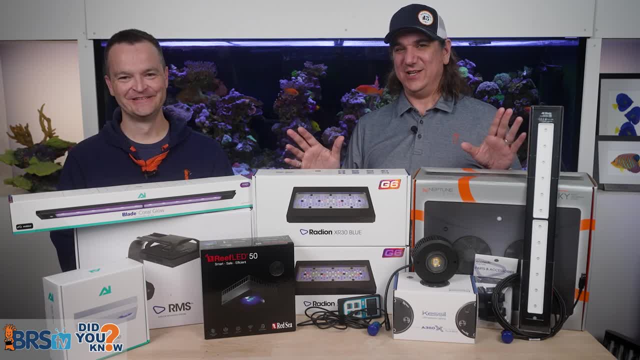 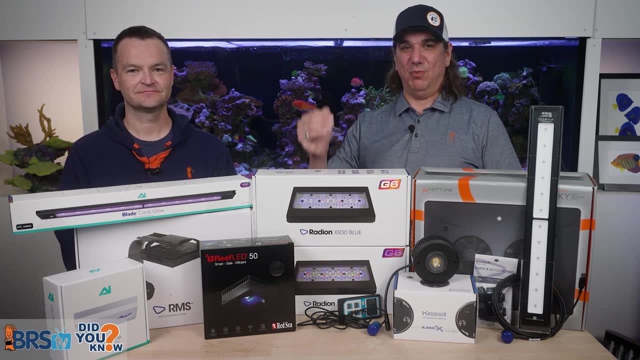 Nobody, every nobody, is spacing them 24 inches apart. So like if you go, look, just go go to. if you want to know what people are doing for lighting, go to Reef2Reef and find the tanks of the month. 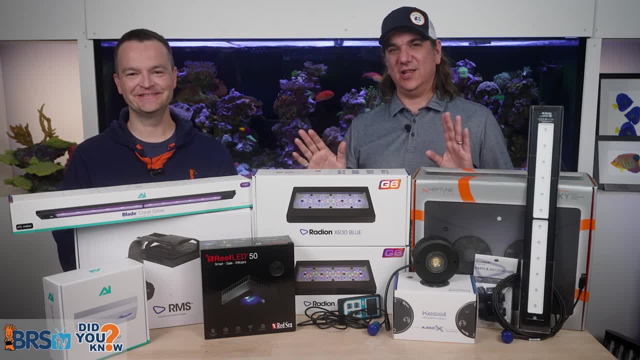 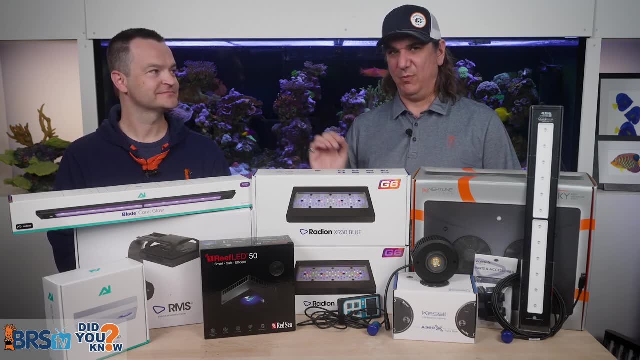 and just look at them one after one. Not a single person is doing it that way. So 12 to 24 inches will be your best bet if you're going to go with these Really easy to install modular lighting. Number six, the second approach here. 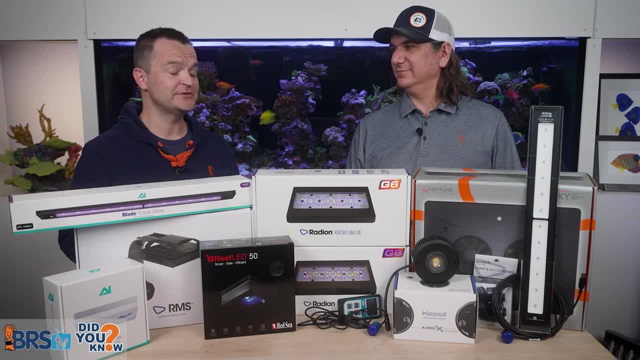 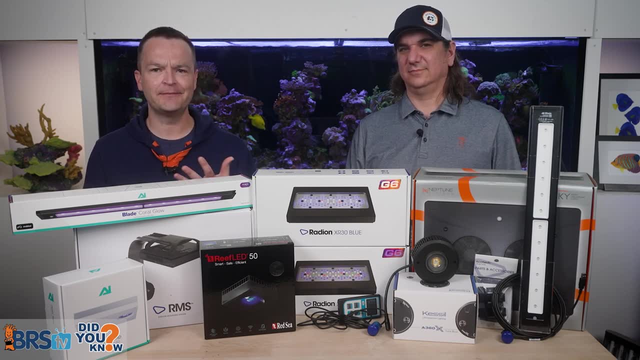 are large panels or fixtures And, honestly, these should probably be more popular than they already are. We're talking about the Orphic, the ATI, Stratton Reef, Breeders Bank of T5s, Phillips, Coral Care and Neptune Sky being some of the most common. 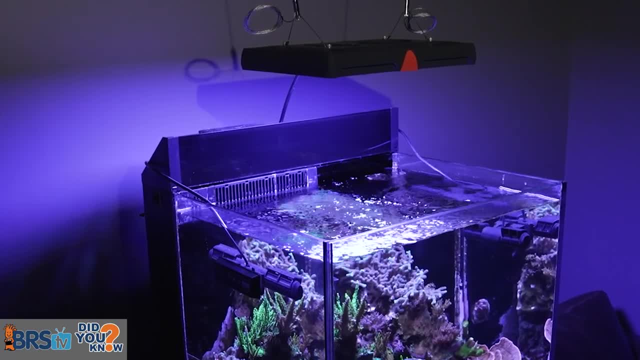 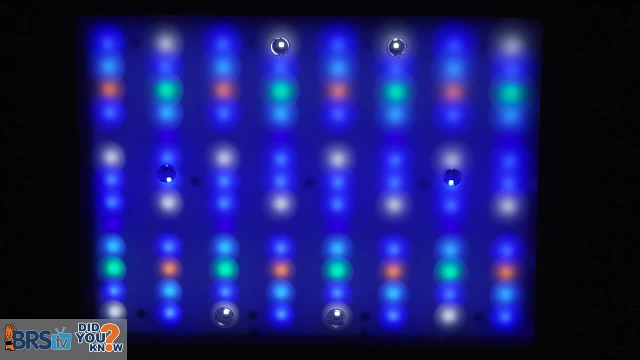 Yeah, these are large light sources that wrap the corals in light, with fewer told modules, which means in many ways they're cheaper because they can actually be the same amount of LEDs and the same cost to cover the same area, In which case now, like one every 24 inches. 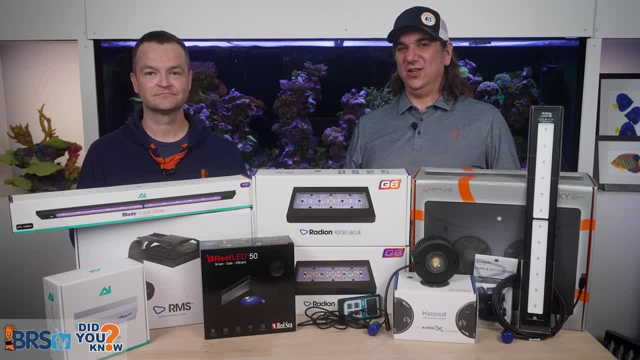 is very legitimate. Okay. the reason, though, that I think that they're not that popular is because they're big in a world like small, And you just don't know any better until somebody, like, really really drives it home, and the bigger is better. 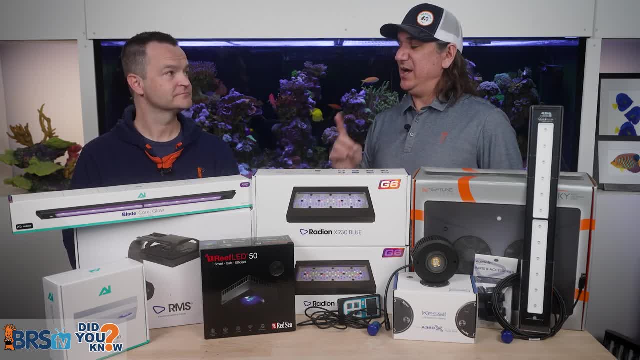 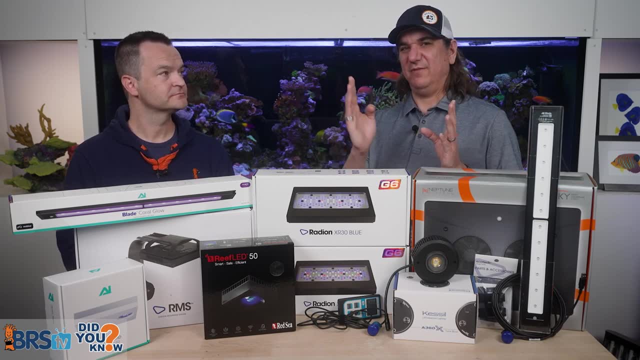 You're just not going to do it. And the reality is some people actually might know bigger is better, But would prefer actually just to achieve that through more small ones. They know, and that's why they're willing to invest in one every 12 or 18 inches instead of these big guys. 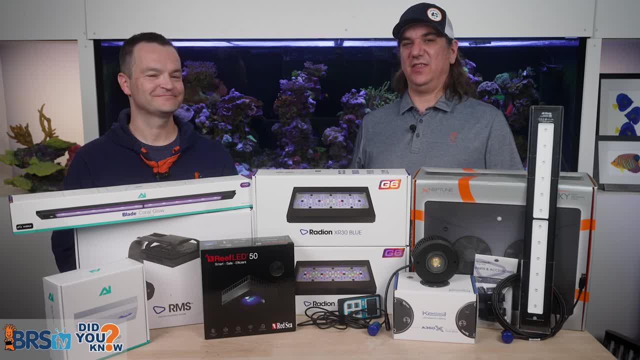 Okay, but I think the real reason gets back to that thing. The number one determining factor for most reefers is how easy is it to install, And most of the ones that you just said are kind of hard to install. Like you're going to have to drill holes in your ceiling. 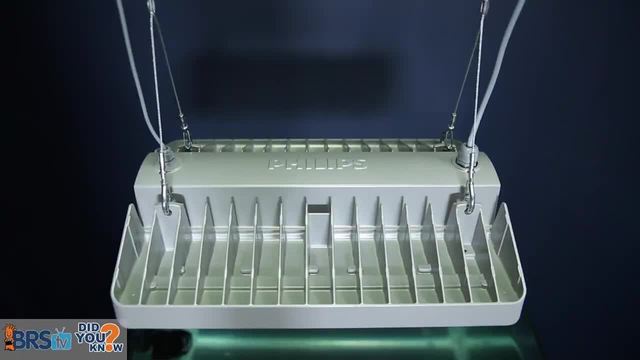 You're going to have to. they don't really come with like leg mounts and stuff. I mean the Phillips Coral Care which, like, really should have been one of my favorites. Yeah, And one of the big winners is, you know, 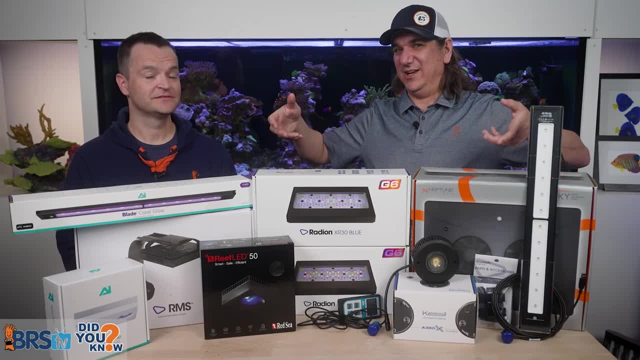 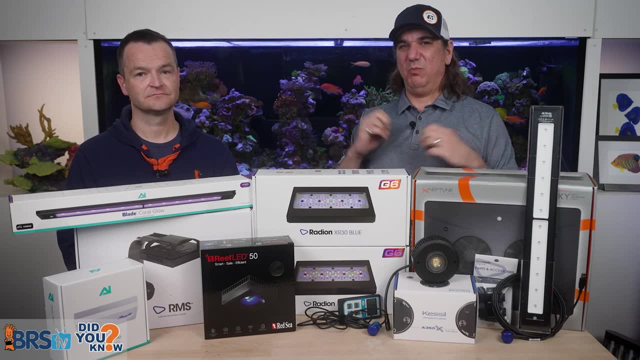 I think it's like 20 some pounds. you know it's in the neighborhood anyway. it's heavy. It doesn't have a bracket. I had to figure out how to mount it And right then, a whole bunch of you just checked out. 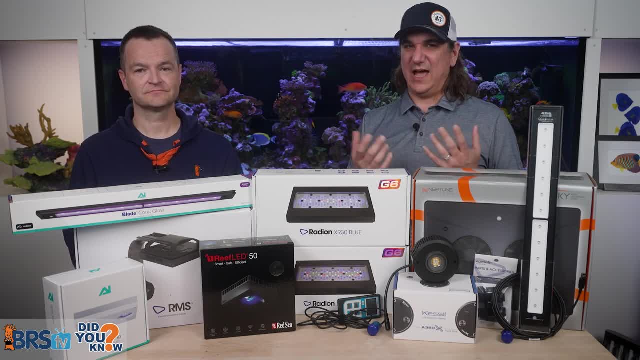 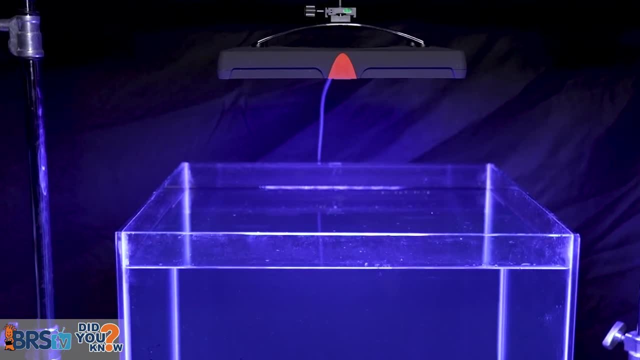 because that's just not right Now. the one exception to that would be the Neptune Sky, which happened to be smart enough to loan the bracket fitting from the Radion, which is interesting, But you can now use just the bracket kits that are already there. 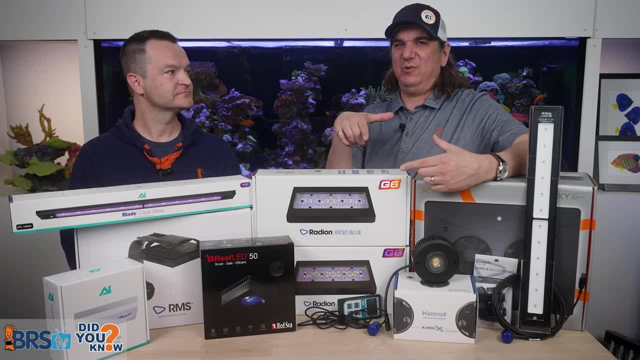 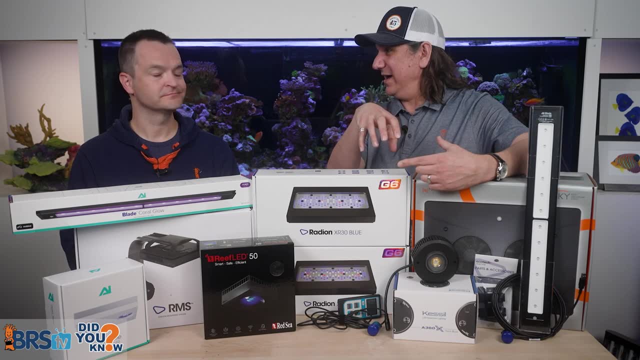 They have like a same whole pattern And I guess I would tell you that when I talk to the people there that they said that they would have liked to see this pole pattern become the universal pattern. So the mounts out there work for everything. 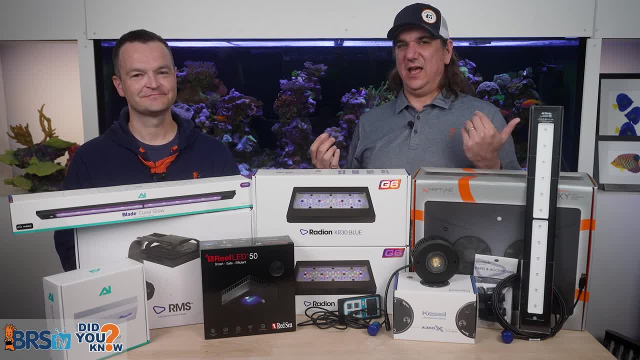 If you'd like to see that, let everybody know. But outside of that, like most of them are really hard, Neptune one being one of the outliers in there. these big modulars should be more popular than they are, but really the reefers just haven't adopted them. 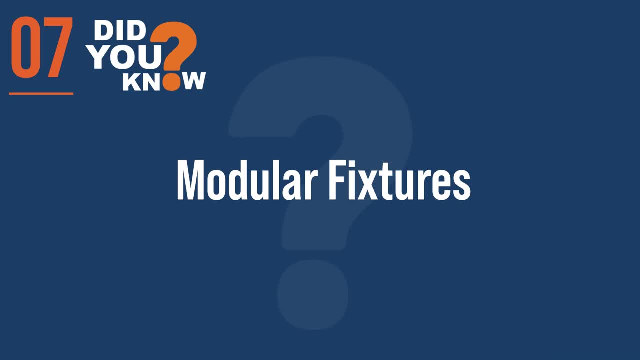 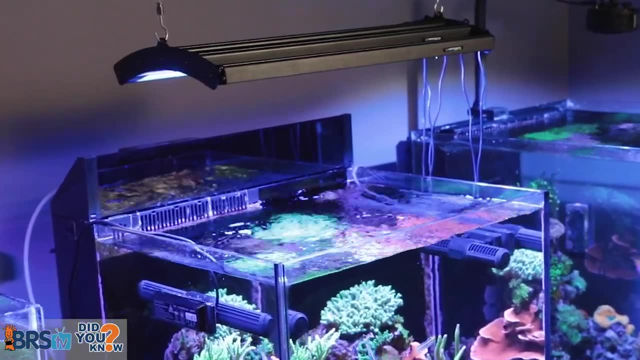 at large scale yet. Number seven, the C-Series. The third approach to achieving that end-to-end light are modular fixtures. These are just light bars that you put together and you combine them to create one large fixture. We're talking about the Reef Brights, the Orfex. 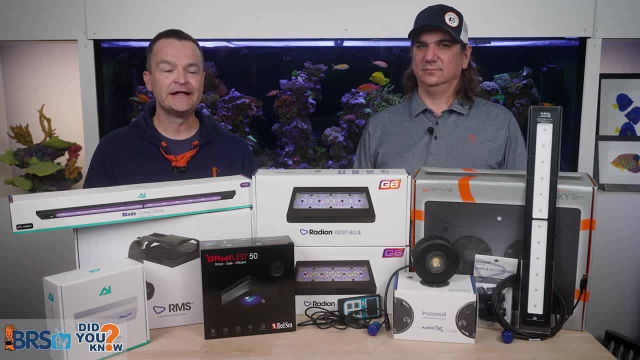 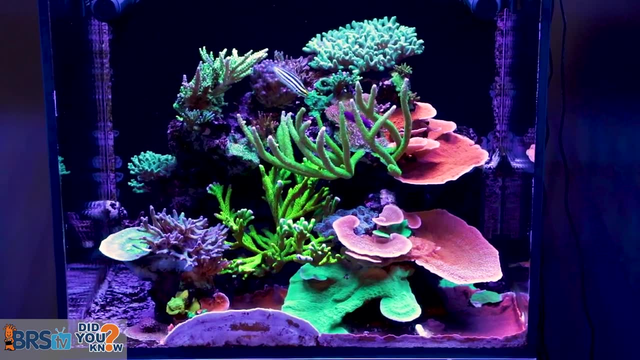 and the AI Blades are some of the most popular and the most common. The benefit here is you achieve end-to-end light that absolutely wraps and envelops your corals in just a blanket of light. Some of these are also really easy to mount. 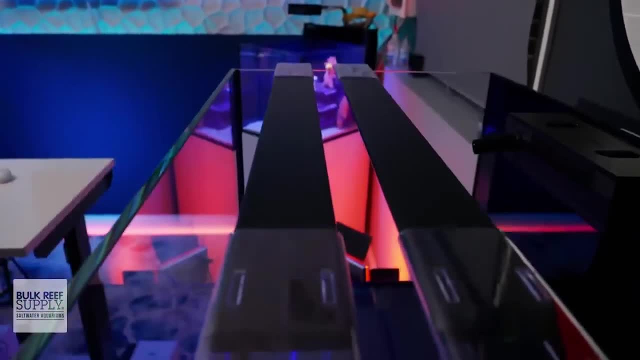 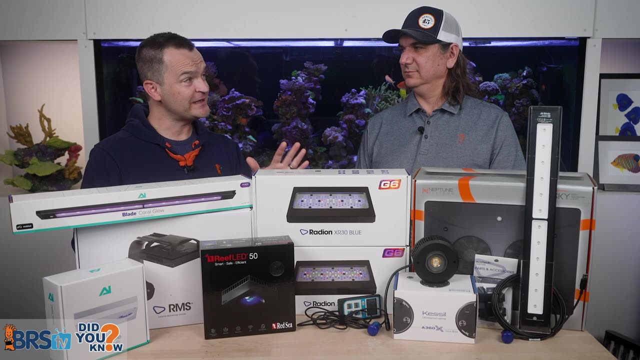 The AI Blades, for example, can either be mounted just directly on the top and the edge of the glass, or it comes with some legs that can raise it up a little bit. I'm betting something: that these will become the most popular way to do lighting as the hobby evolves. 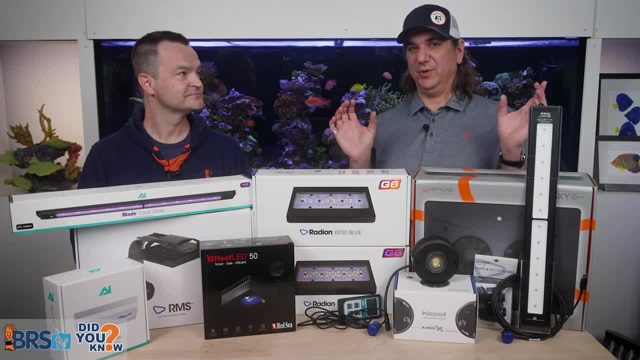 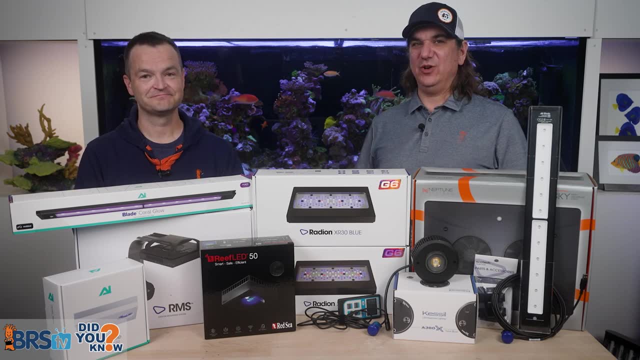 My first experience with this was actually they sell a little bracket. we can bolt a bunch of Reef Bright XHOs. When we built those together and put them on the E170, everybody in the room said: why have we never done this before? 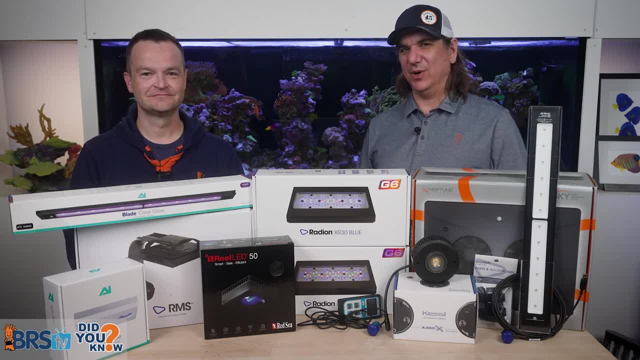 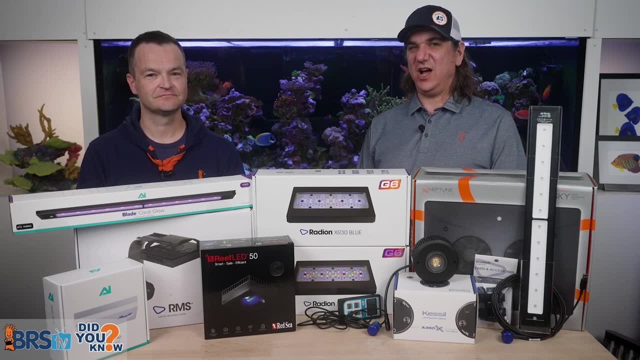 Why is this not more popular? Because this outperformed most of the things that we tested. Okay, so I was really really shocked at that point because it did really really well And like it's all those things, like you know, the fixtures. 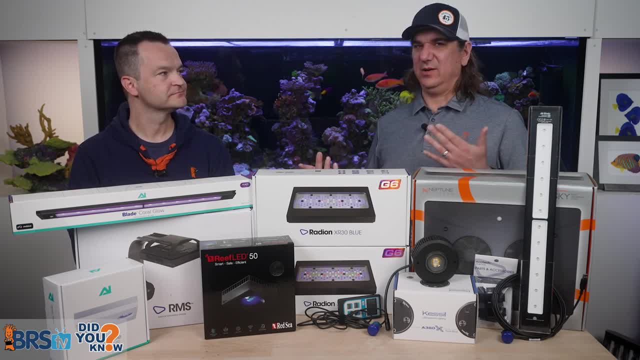 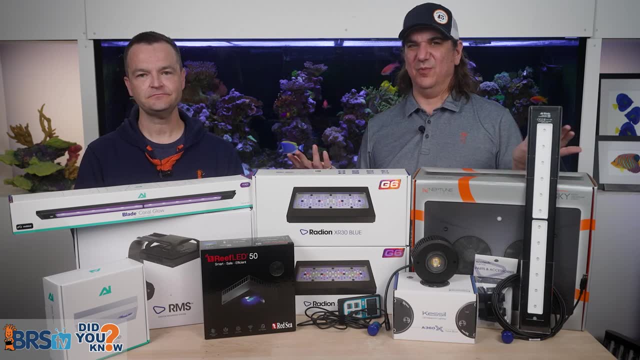 like part of the problem that fixtures like big ones aren't really popular is because they're really hard to distribute, Like like. fish stores don't want to stock every available size of all this stuff and you guys aren't buying it, So it just doesn't make any sense. 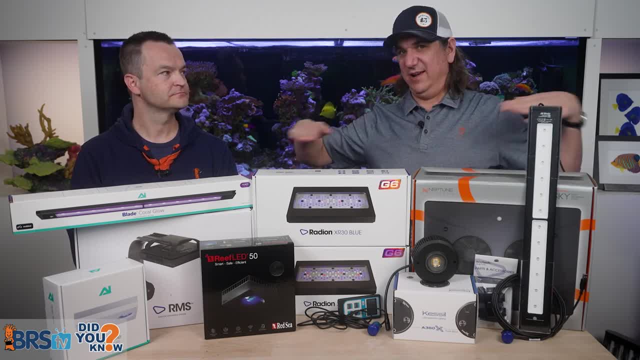 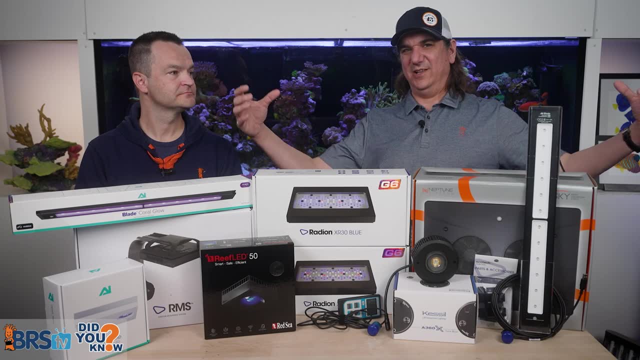 These things, like these little blades that like, like you said, just rest right in there. I mean, the mounting doesn't get any easier than that. And then the legs are optional. You can buy them afterward and they just go a few inches. 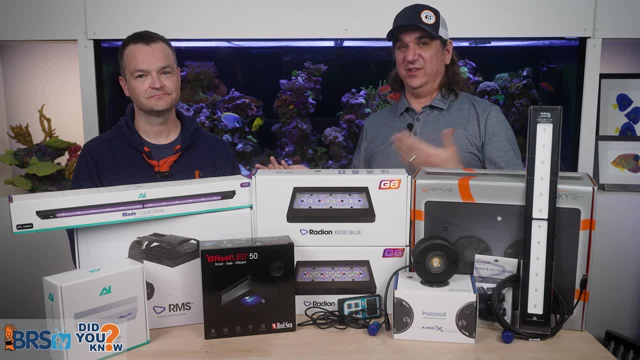 and you just set it right on the top. Doesn't get easier than that. And if I just put four of them in there, then it's the same thing as a fixture. In fact, what we used to think about as T5s is a fixture. 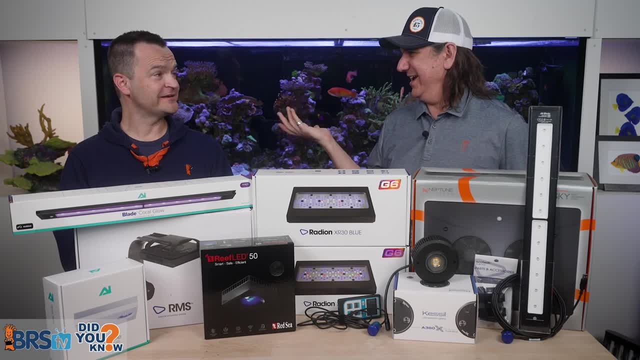 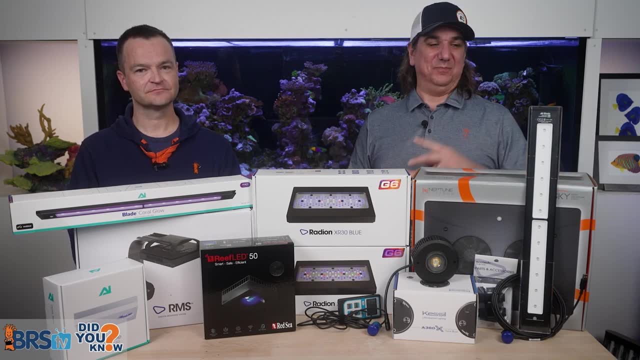 but really it's eight light strips. You know, each one of those balls is just a light strip, And so it's really just kind of recreating that kind of thing. I also agree This is super, super easy to install, And now that the lights that are coming out, 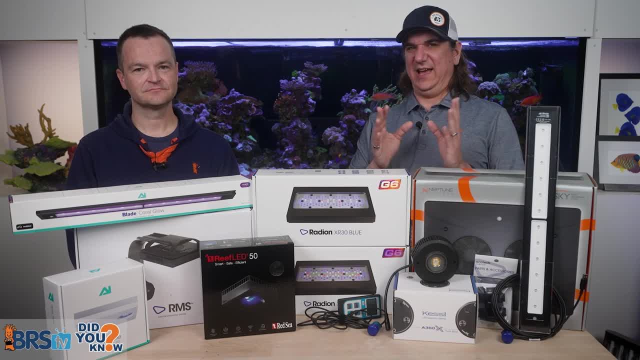 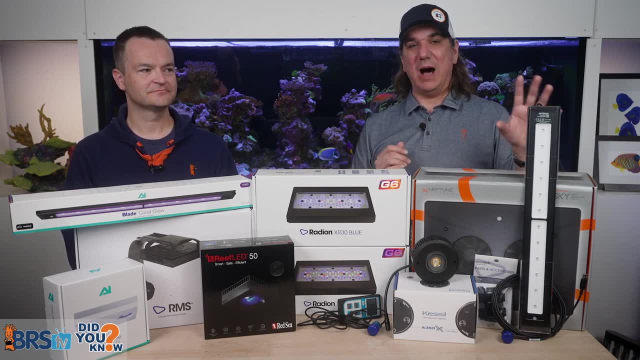 aren't just limited to, you know, creating a spectrum that is designed to be like supplemental. They're now designed to actually light the whole tank. This will probably be one of the more popular options going forward, because it solves so many needs and it's easy to install. 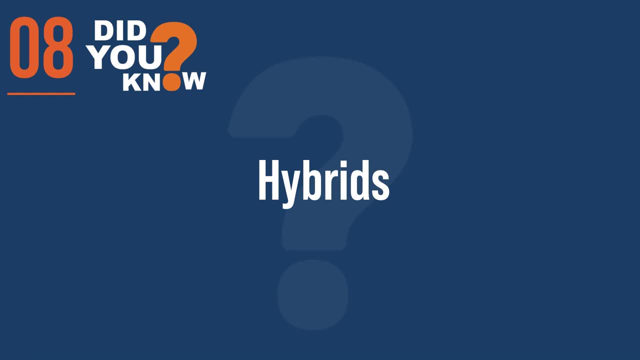 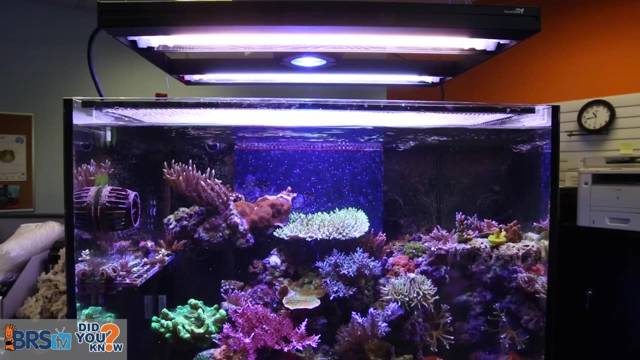 Number eight. the fourth option for achieving that end-to-end light are hybrids, The most popular being a three-point hybrid where you take one single point of light that emulates the sun and then it is flanked on the sides by larger strip fill lights. 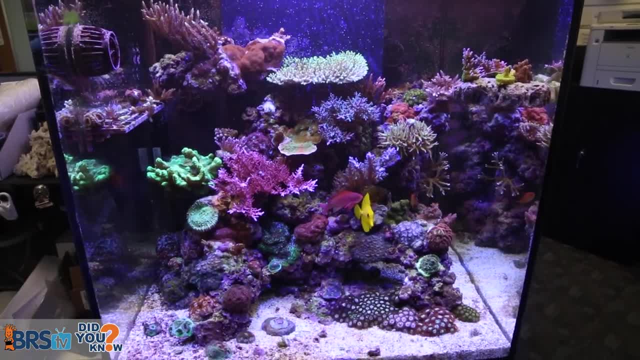 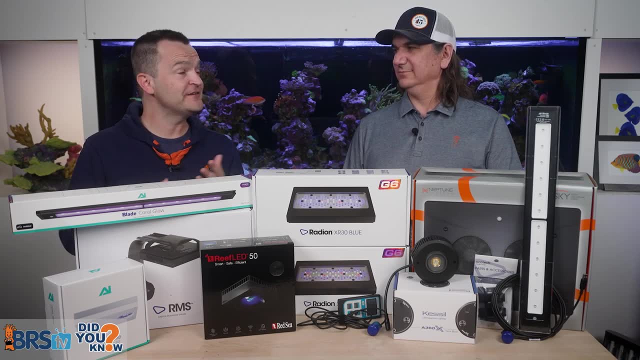 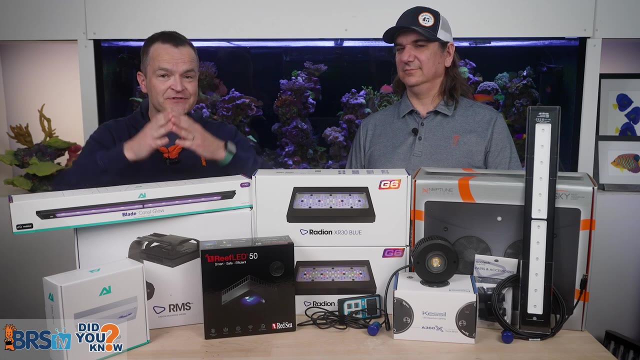 which emulate that blue sky kind of filtering all that light and enveloping that coral. This is often a cheaper way to do things, with better shadow reduction and even more spread, than the modules alone. Also, if you tend to already have one, one of those smaller modules, 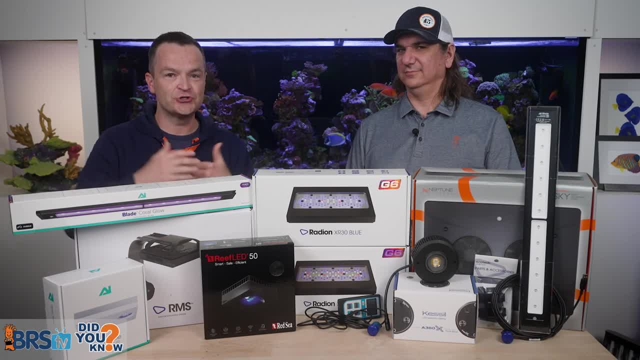 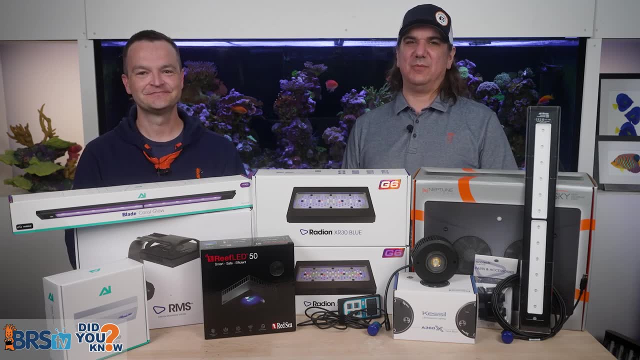 you can upgrade by buying a couple other modules. You don't have to go out and buy something completely new. Finally, we get to talk about my favorite option. This is my favorite option for a couple of reasons. One: I really like the idea of emulating the sun. 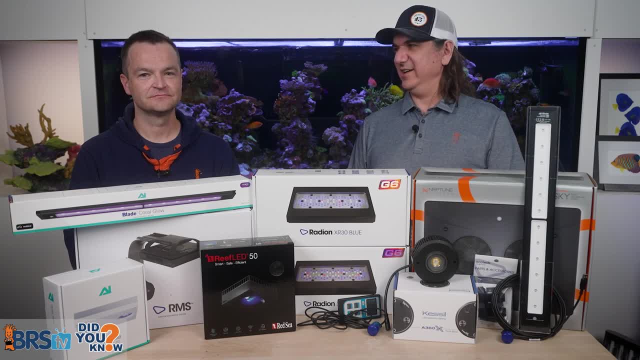 and the sky at the same time. Two: all of my best tanks have been installed this way, with one exception. The 750 XXL is Radeon spaced every 18 inches. That one has actually done phenomenally well, But other than that one, almost all of my tanks have been. 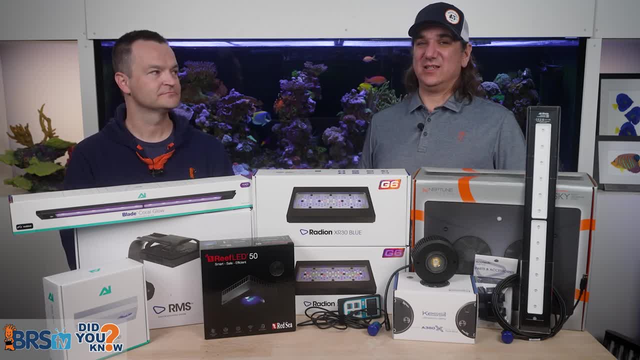 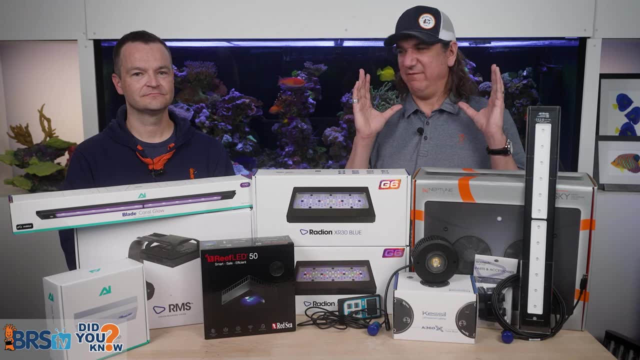 three-point lighting solutions, And one of them is because I care what it looks like. I want this tank to come alive. I want to see the shimmer. I want it to look like when my face is down in the water snorkeling or diving man. 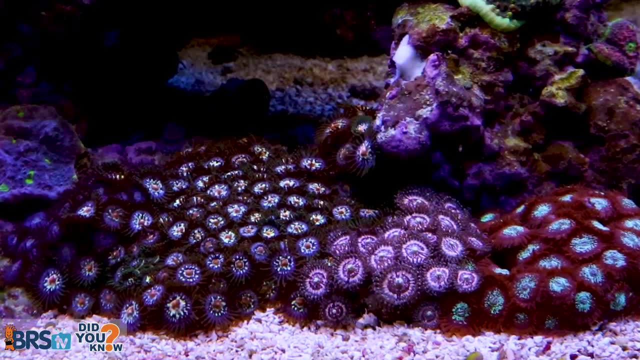 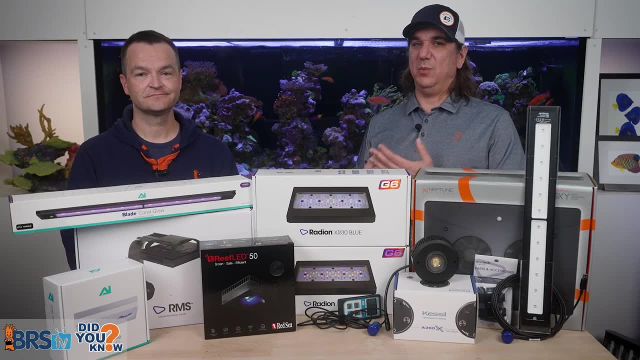 I want to see that rhythm and movement come to life, And there's just no way to do it other than creating that single point of light that you can kind of tune the shimmer to exactly where you want it. So some of my favorite options would be like the Kessels. 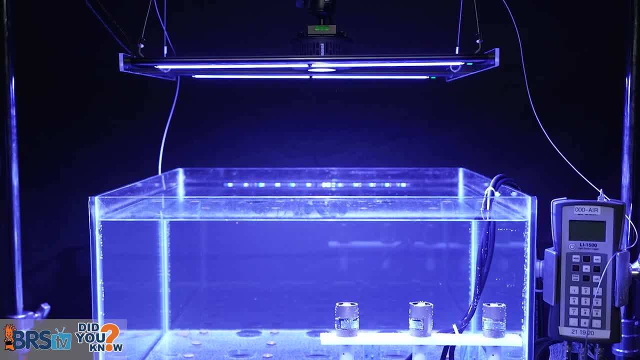 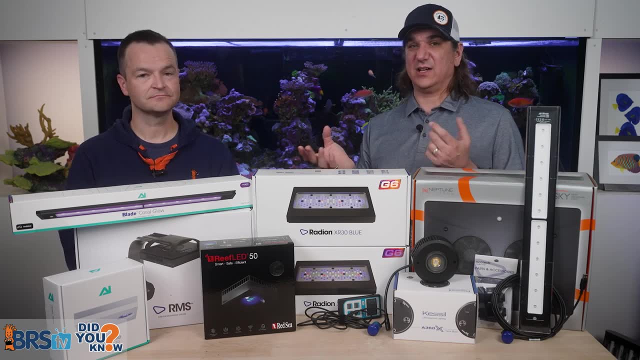 that are paired with something like the Blades. We've done Kessels and T5s many times in the past. You could do Kessels or we could do Radeons, like the XR15 matched with the Blades. In that case, in our testing, 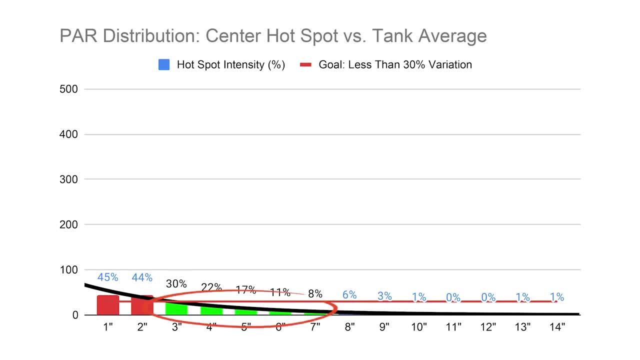 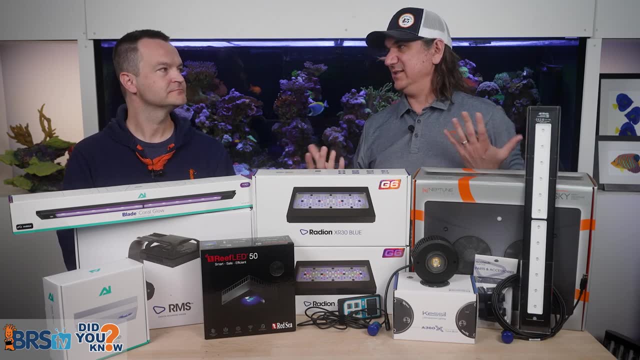 we actually found that this thing had a really huge sweet spot. It was super even That ultra wide angle light coming out of the wide angle module. then filled in with the Blades, it was a really awesome solution as well. So the really cool part about this one. 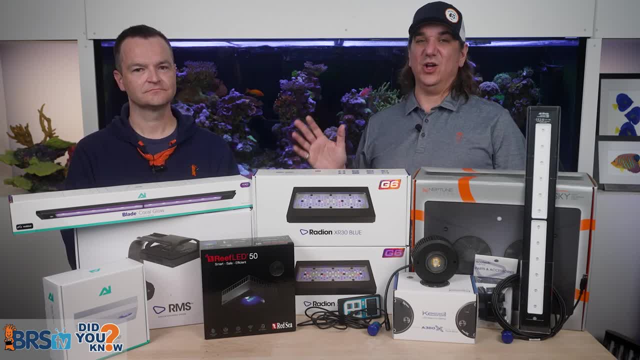 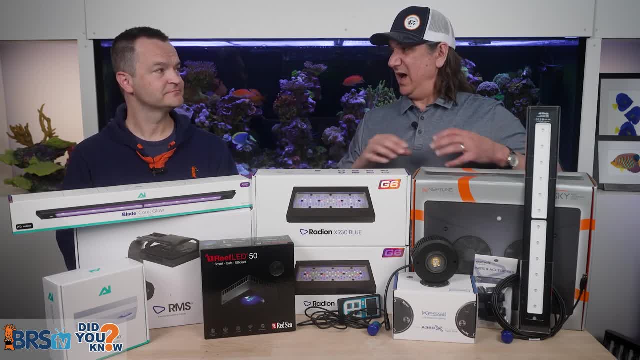 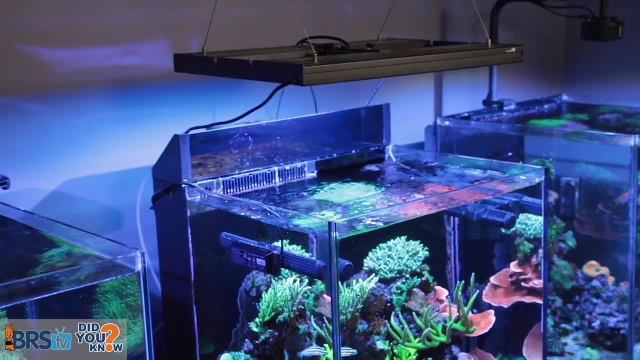 This is a case where, if you already have modules, man, I can just throw those strips in and I can upgrade what I already have to today's standard, which makes it one of my favorites as well. I always said we were gonna do eight things. 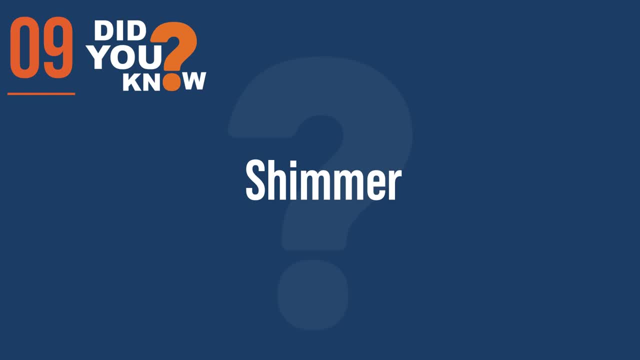 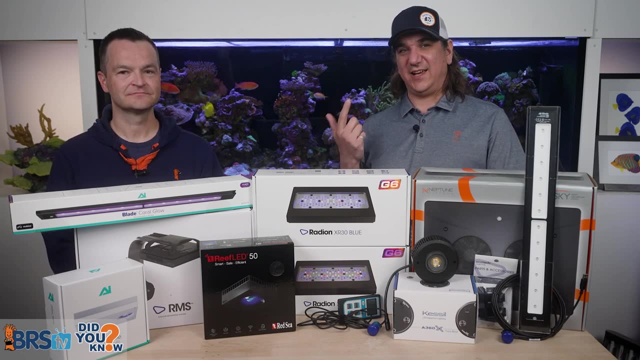 but we're actually gonna do nine, because I just talked about shimmer and I'd love to share a little bit more because you can actually know what you're going to get ahead of time as well. There's five types of shimmer. There's disco, TV static. 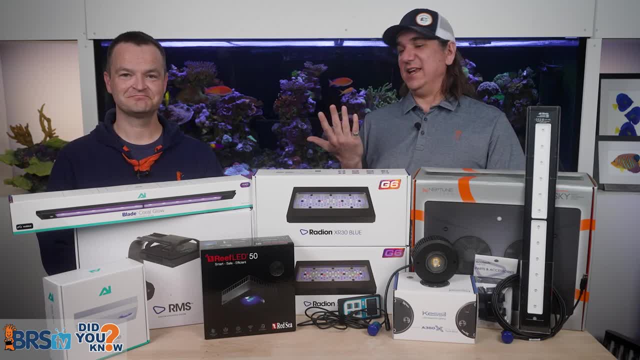 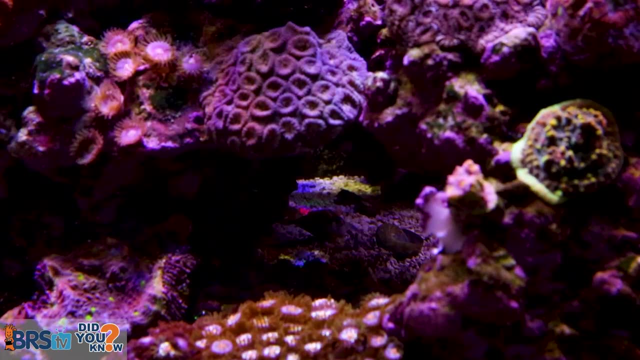 cross none and what I would call perfect And you can pick any one of those things. So disco is actually when you see like little bits of color shooting all over the place like a disco ball, and you just see red and green and all these things. 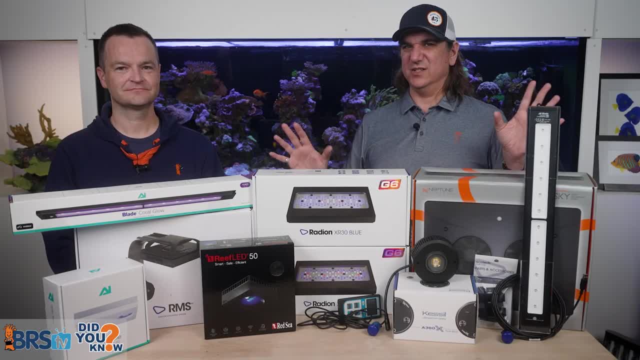 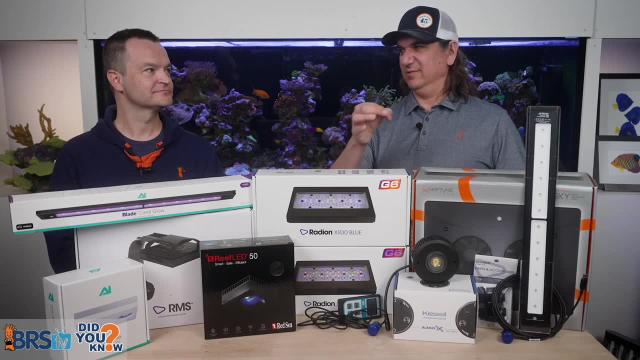 just shooting around all over the tank And it doesn't look like shimmer. if you look close it just looks like things are going crazy Random color. Yeah, Okay, so you can know ahead of time. it's because they're using these like lenses on there. 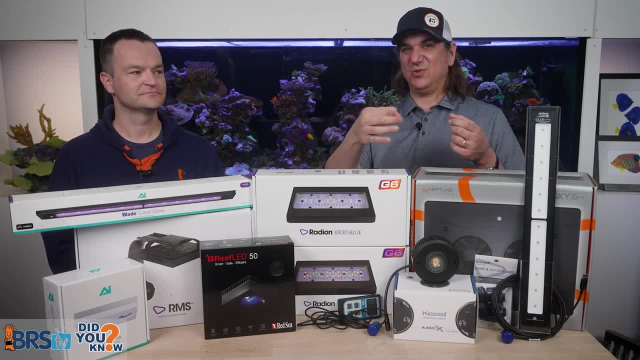 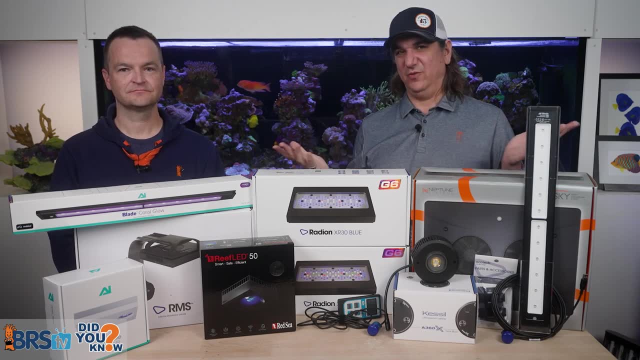 Each LED has this pretty specific focus lens on each one And what that does is creates a beam that reflects off of the little ripples on the surface of the water, shoots these colors all over. So if it has those lenses, specifically these lenses that like are like really common. 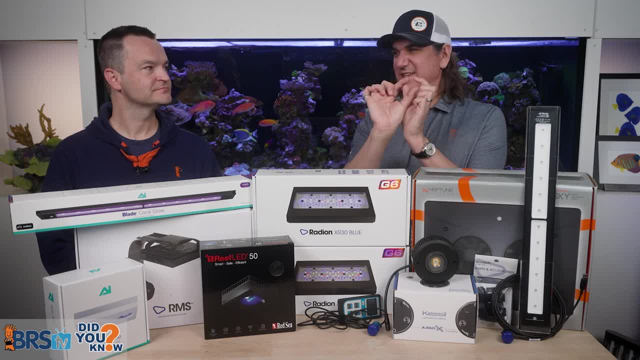 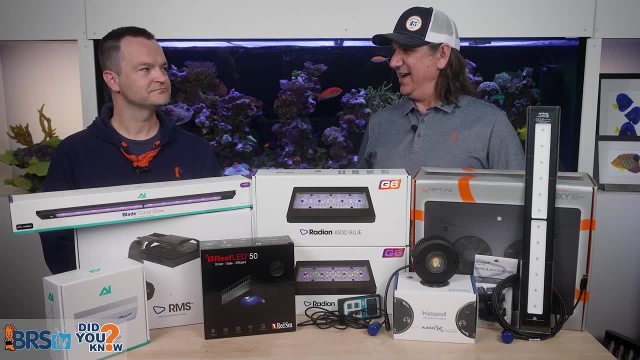 in commodity like LEDs or like these little round discs. you know, if you see those things on it, I know for sure it's gonna have disco. There's another thing called TV static. This looks more like that fuzz like when you used to watch like analog TV and go shh. 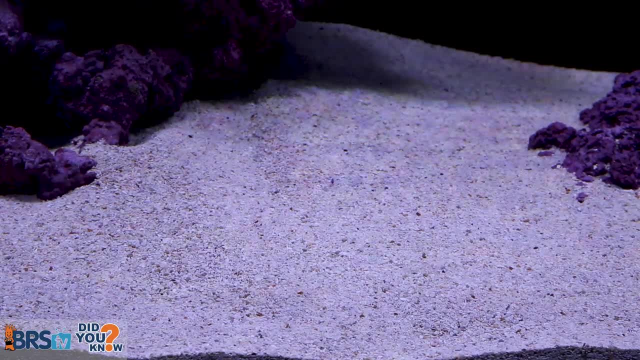 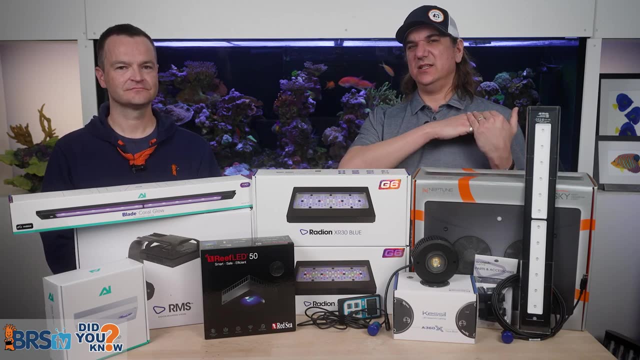 Oh, I don't know if any of you guys even remember that anymore. It also almost looks like little ants running around the tank And it's like this fuzz on the tank. Okay, that is created when you have tons and tons and tons. 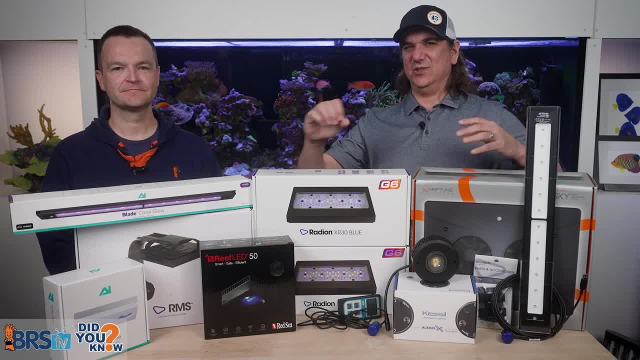 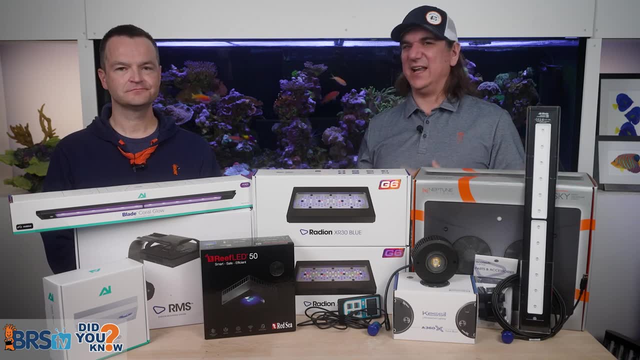 of low power LEDs, right, And so there's just all these little points, and there's so many of them that it has a little bit of movement, but it looks more like fuzz or static than anything. There's also what I call chaos, chaos shimmer. 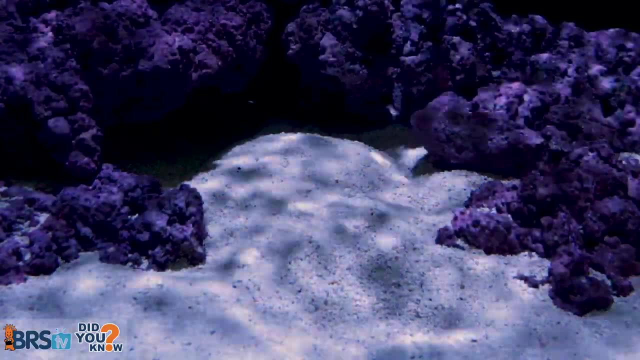 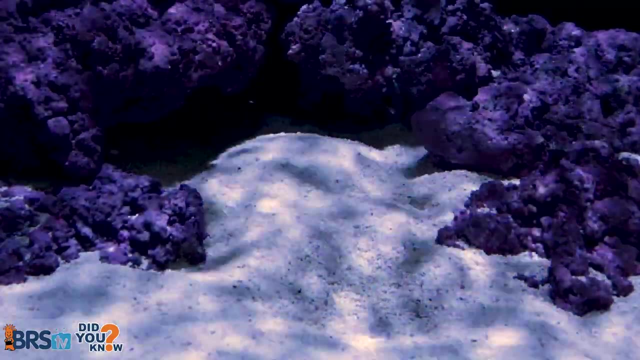 So this is the Kessels alone for me, which is just the one Kessel by itself Or a single point of light like that. And then if you have a bunch of those Kessels, there's just so many sharp lines because there's no skylight kind of filling in. 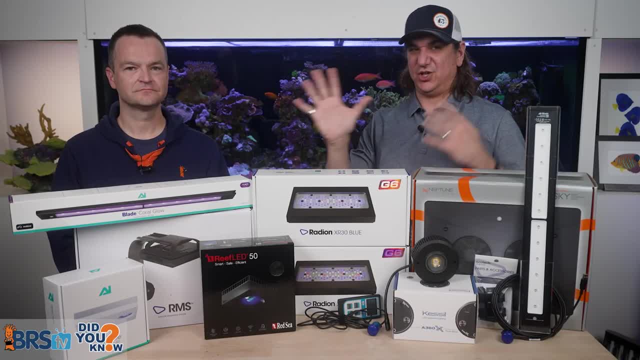 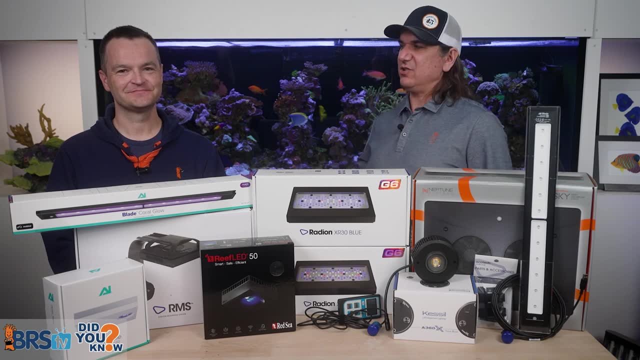 or buffering it, And so what it does is it just looks really sharp and there's just like a lot of rhythm and movement. Some people will love it. For me it's just a little too much. There's another kind of shimmer called none. 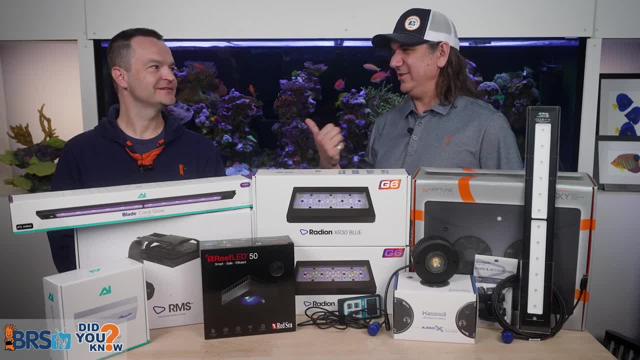 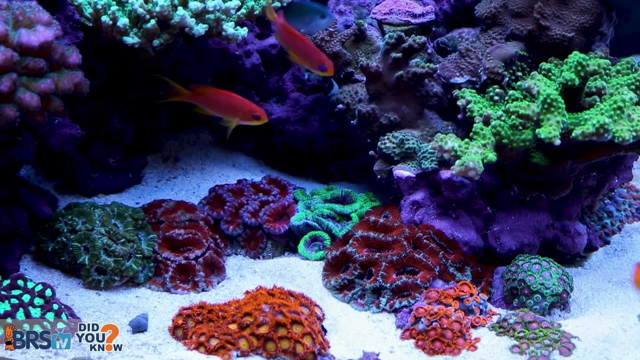 Oh, a none. Yes, Can you tell me what none looks like a little bit to you? Yeah, none is literally when you look down and you don't see like any movement on the bottom. It's usually what? Oh, just a large like bank of T5s will accomplish that. 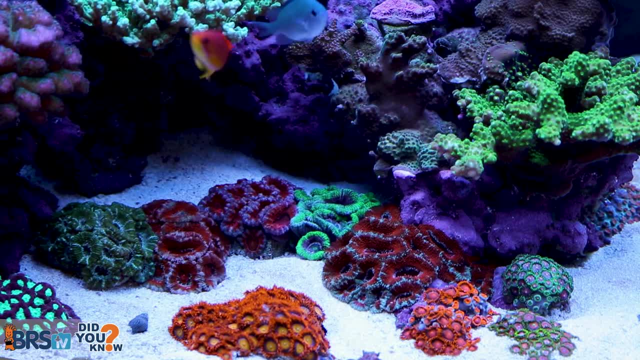 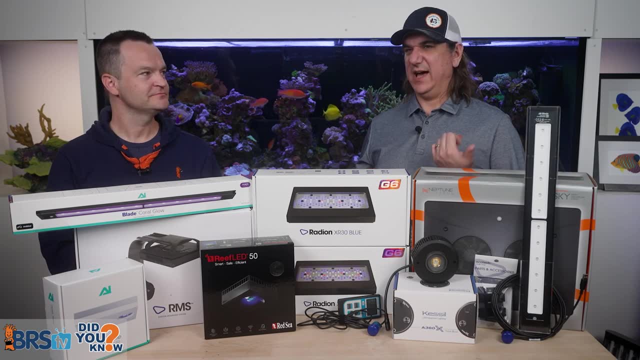 where there's not a single point of light and you just look at it and it just looks beautiful, but you don't see any shimmer. Diffused lights will do that in many cases too, So, like the sky here, will do that Anything. you kind of put a diffuser on. 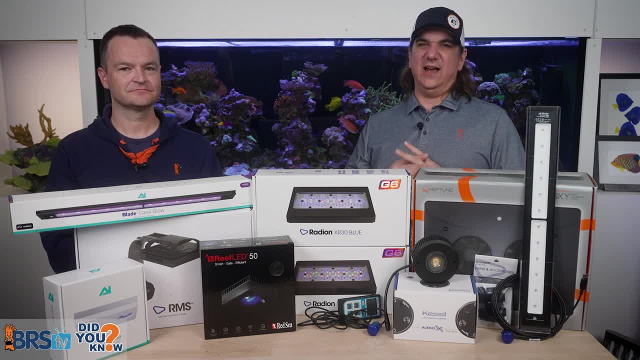 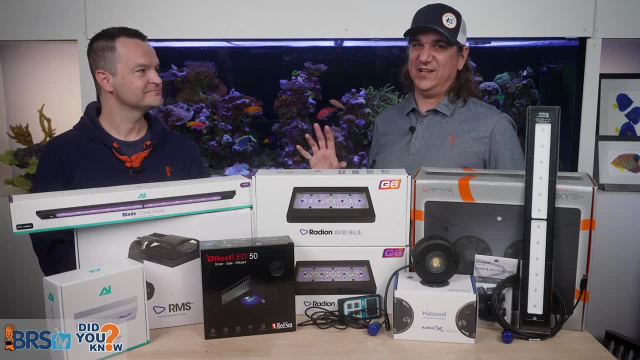 will mute the shimmer a lot And the way that everybody describes it is a tank with shimmer. looks like you're snorkeling. You got like a little piece of Fiji sitting behind you in your house. A tank with no shimmer looks like a picture of a reef on your wall. 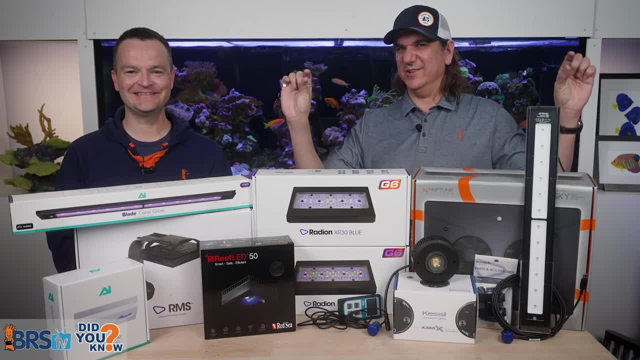 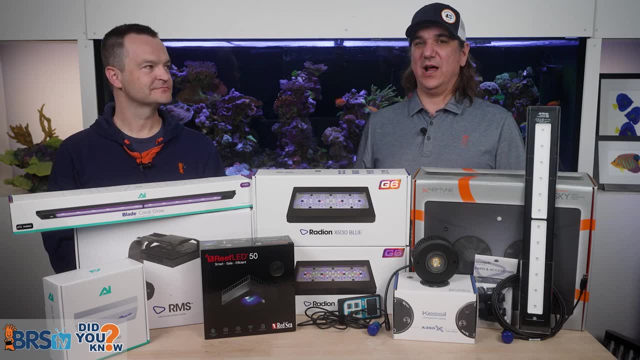 Yeah, that's pretty good, And almost like the fish are just kind of like floating in thin air in this picture It lacks like an element of the environment that it was really in. The last type of shimmer is one I would call perfect. 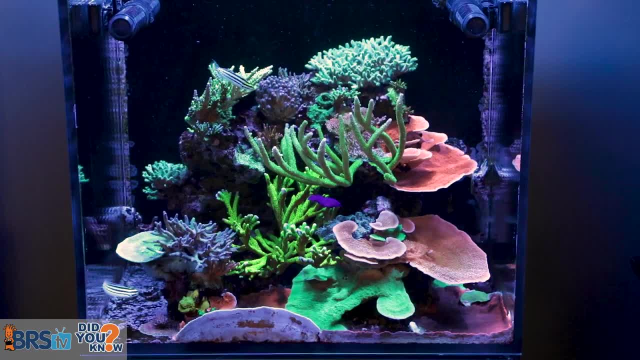 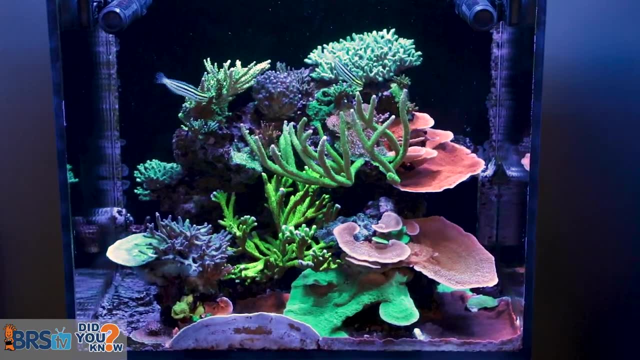 So perfect to me means single points of light like. the Kessel is one of them. I bet you the Red Sea would fit in this pretty well. The XR-15 fits in this pretty well, but single kind of more compact sources of light. they create a lot of shimmer. 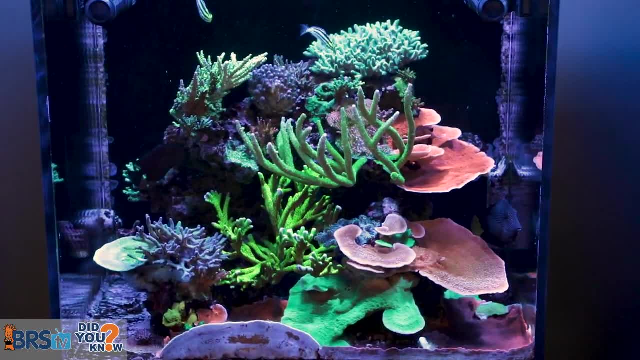 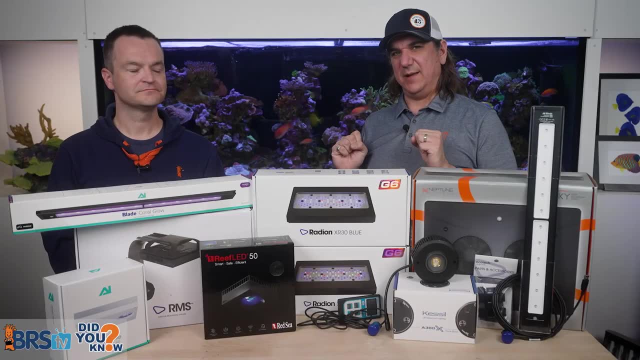 And then the fill lights of the sky in there on the sides, providing that like kind of atmospheric blue light on the sides and things. Now, what it does is it softens the shimmer right And now I can actually tune it So like with something like the Kessel.